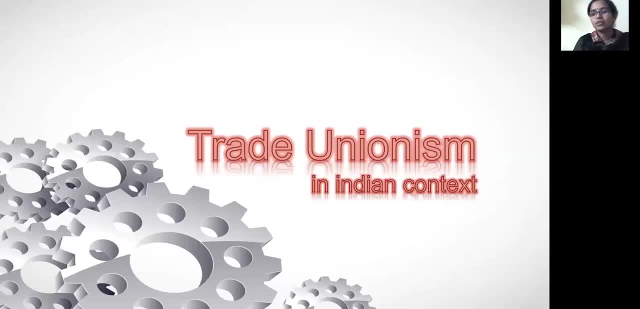 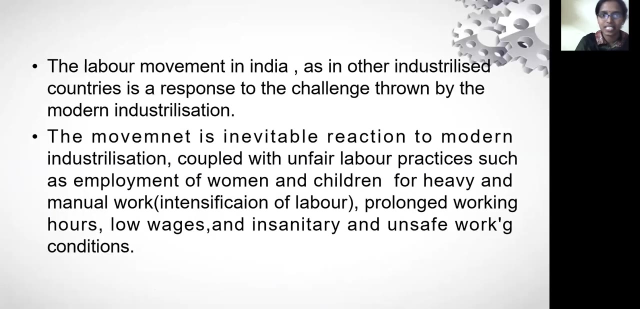 Hi everyone. today we are going to see the trade union movement in India and various trade unions in India and structure of trade union. So the trade union in India. to discuss about the trade union movement in India, first of all we have to talk about the labor movement in India. 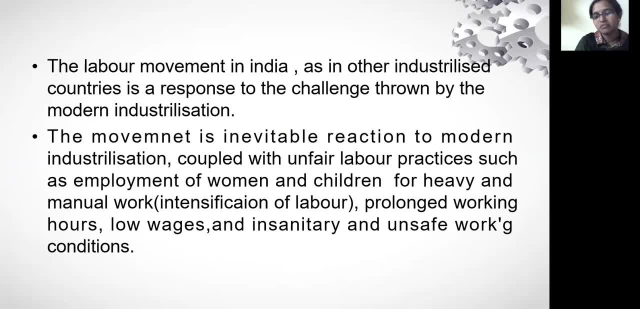 Because the labor movement is an early stage of trade union movement. So the labor movement in India has been started, as in any other industrialized countries. It is a response to the challenge thrown by the modern industrialization or the modern factory system of production. 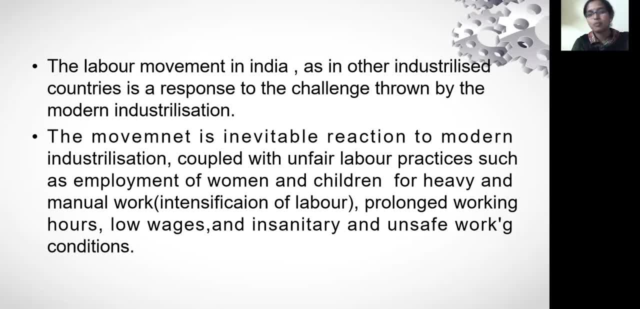 So the moment is inevitable. this labor movement is inevitable because it is a reaction to the modern industrialization which has been coupled with the unfair labor practices such as employment of women and children for the heavy and manual work, and intensification of labor. 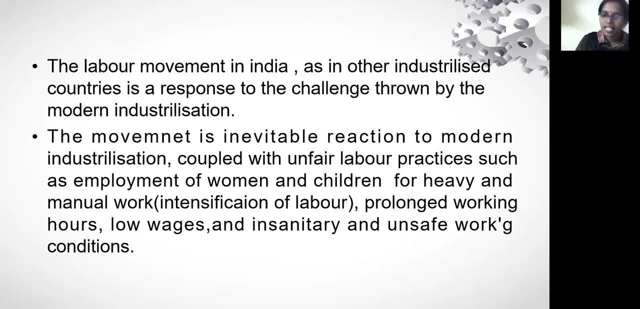 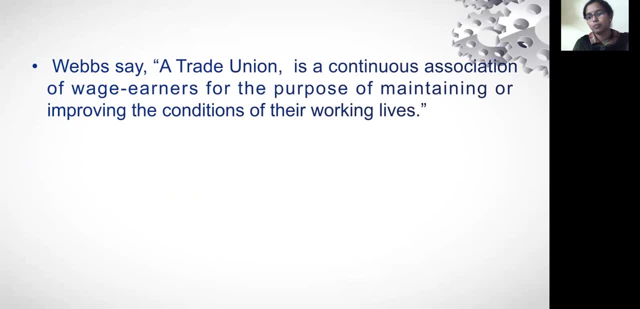 Prolonged working hours, low wages and in sanitary and unsafe working conditions. These are the causes of the rise of this labor movement. So let us see what are the basic definition of trade union movement and the labor movement, or a trade union and labor movement. 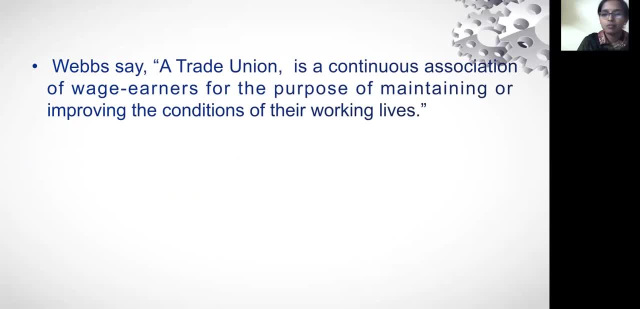 The trade union and the labor movement. The labor movement is for the labor, whereas the trade union is by the labor. So trade, labor movement is for the labor, For the welfare of the labor. it has been initialized or initiated by the reformist, social reformers or philanthropist in the societies that are non workers. in the society has been revolted against the exploitation of the workmen with the employers. 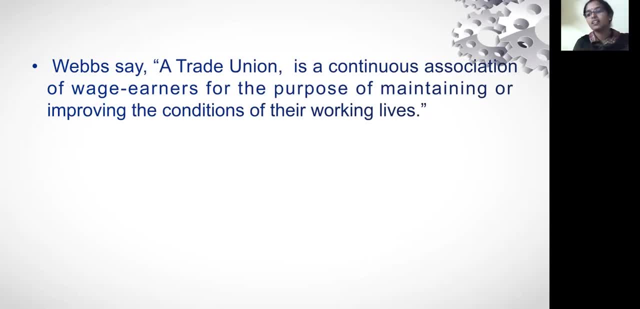 Like Bengal, SS Bengali, who has? who is a revolt? who has started agitation against this? The labor movement is for the welfare of the labor, against the unfair labor practices, against the unfair labor practices, for the welfare and well-being of this workers. on and in the similar way. this trade union is nothing, but it is formed by the workers itself for their own welfare, to protect their own interest. 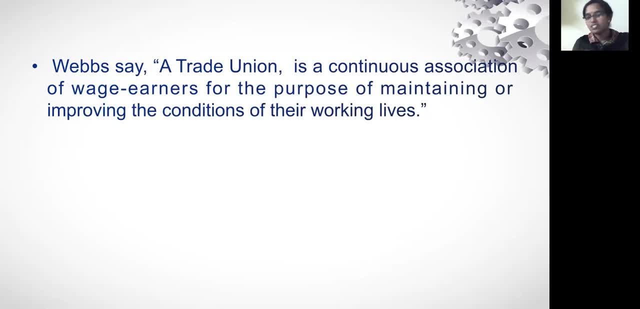 So that is the basic difference within labor movement and the trade union movement. Let us see some of the definitions of trade unionism: Trade union- So according to Webb, the trade union is the continuous association of wage workers, wage earners, for the purpose of maintaining or improving the conditions of the of their living, working life. 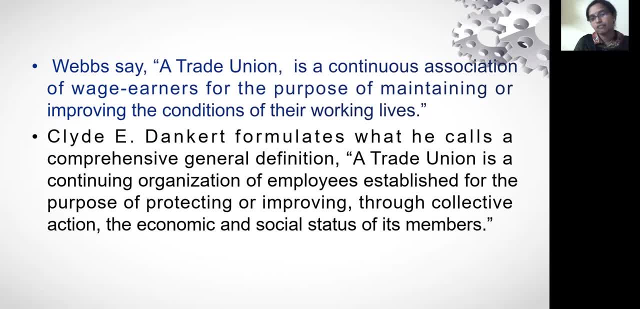 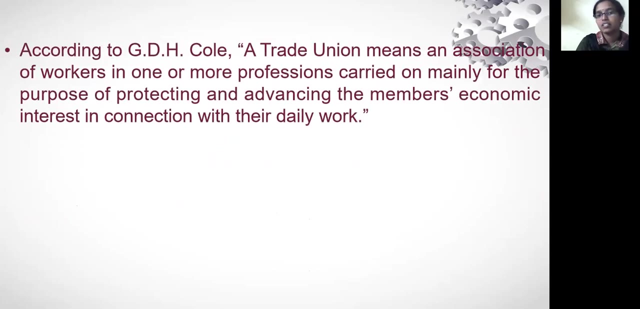 And definition can Denkert formulated or he has given a definition: A trade union is continuous organization of workers established for the purpose of protecting or improving The collective action, the economic and social status of its members. This is a definition which is given and the next definition GHD Kole he has given: the trade union means an association of workers in one or more professions, carried on mainly for the purpose of protecting and advancing the members economic interest in connection with their daily work. 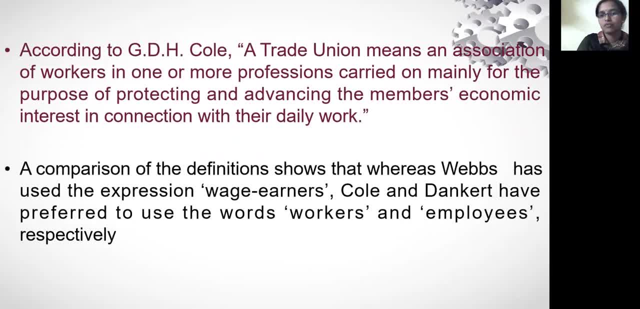 And if you compare the all these definitions, in these definitions we have used, The Webb has used the expression of wage earners and Kole and Denkert has used the expression of workers and employers, employees. all these expressions are are similar, are same. 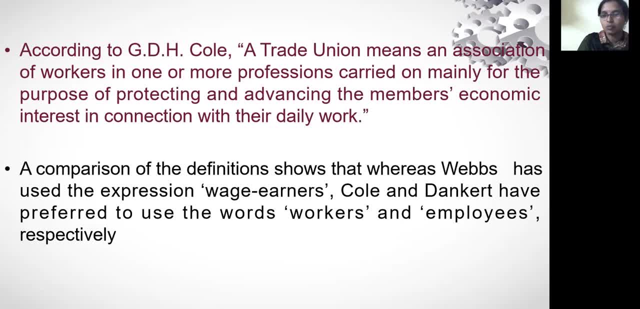 They are, they are targeting to, they are. they mean only the workmen or the labor and the wage. owners and the workers and employees are same, The they have, the, the way of expression, the wording is different, but the meaning is same. 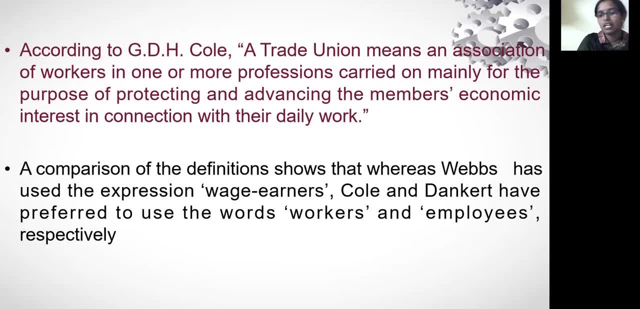 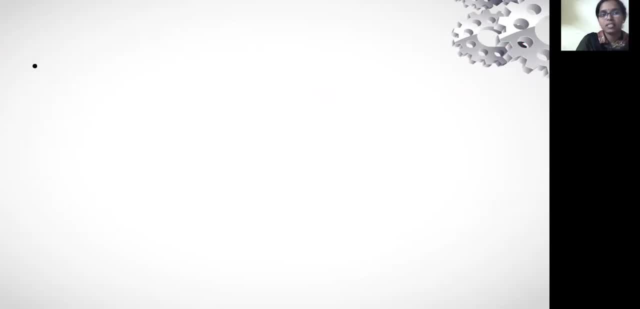 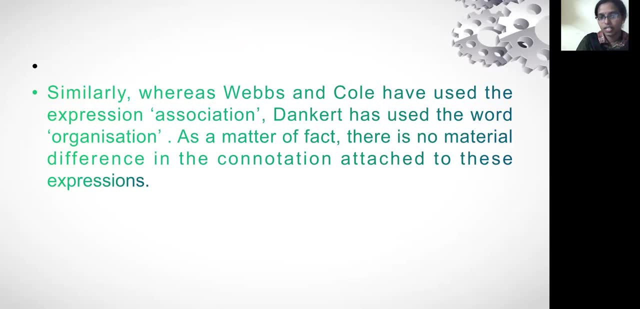 They want to Talk about the age earner. age earners or workers or employees are the same. and coming to the next Comparison, if you see The similarities between Webb and Kole definitions, association and organization, they mean the similar. there is no material difference in the, in the expression or this in the wording which has given by given by this Webb and Kole. they want to see the group or association. they'll be working towards the common goal. 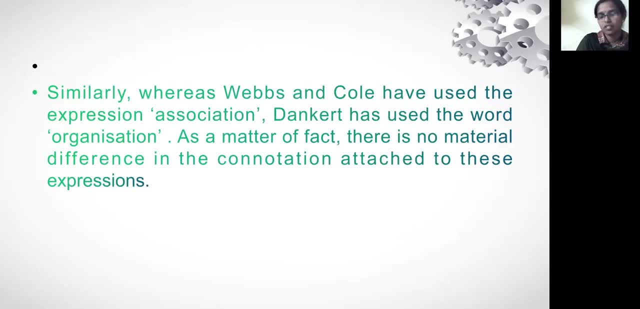 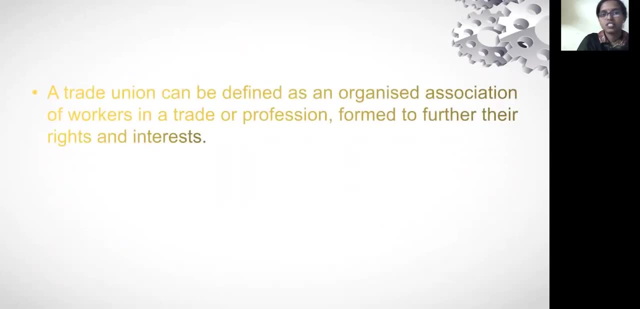 Interest. That is what the association or the organization. there is no material difference between their expression. And the next definition of trade union can be defined as an organized association of workers in a trade or profession formed to further their rights and interests. In India, the trade union was all the trade unions are registered under the trade union sector of 1926. 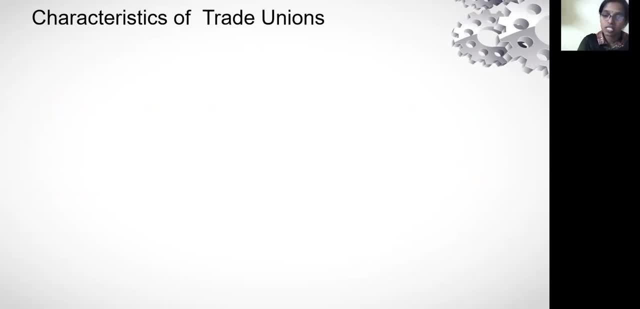 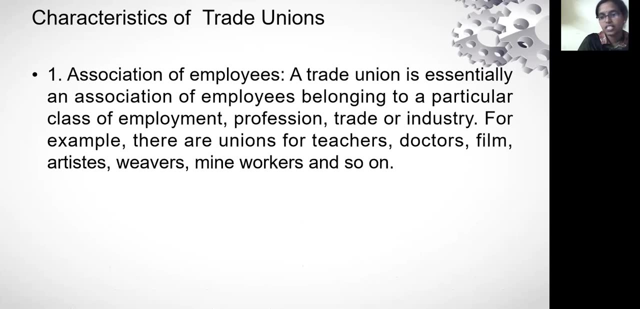 Let us see some of the characteristics Of trade union, then we'll go deep into the history of trade union. Characteristic trade union the trade union is from the definition we have seen. the trade union is an association of employees like, for example, teachers association, doctors association for filling. 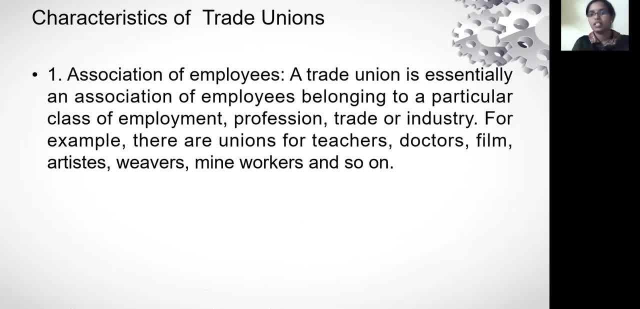 Artists association- where was mine? workers, and so on. The trade union is essentially an association of employees belonging to a particular class of employment or the profession or an industrial Trade. So the second characteristic: it's a voluntary association. Nobody, according to it, is it is joining into any of the trade union. It's up to the 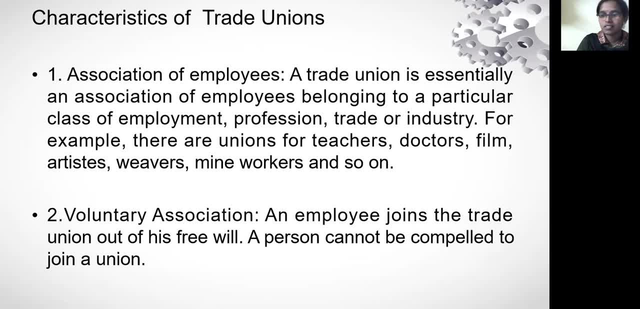 Opinion of the worker or the employee. Nobody is compelled or forced to join any of the particular union. because it is also already mentioned. it was clearly mentioned in the fundamental rights of our Constitution. according to the article 19, to a slowly, we have the freedom of: 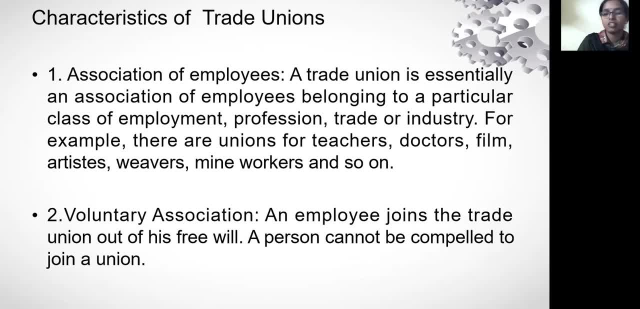 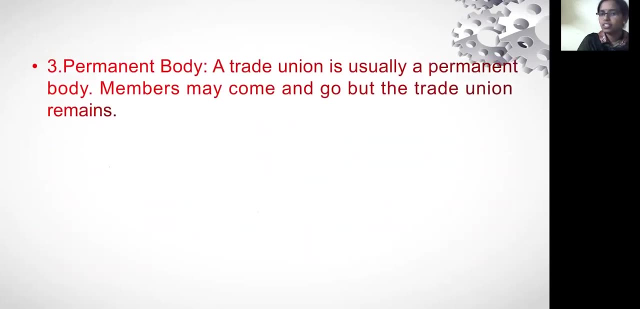 Association. freedom of association means we can, we have all the freedom to any individual as a citizen of India, have have a right or have a right and the freedom of association to join any of the Union as per his will. Nobody is, is cannot be compelled or forced to join any union. And that is the next and the permanent body. a trade union is usually a permanent body. members may come and go, but the union remains. 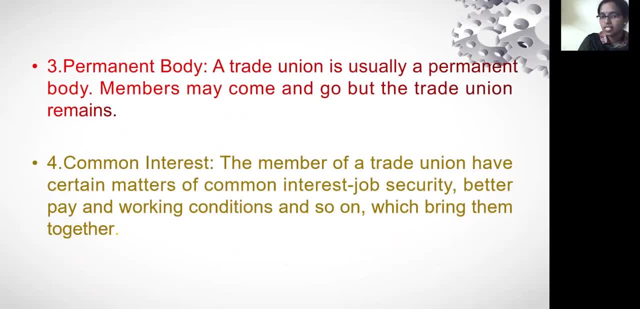 The common interest, the all they will be working towards the common interest, like Job security, better pay and working conditions and- and this is what these are the some of the causes where they form trade union to look of these issues- better payments and job security and all this. next definition is collective action when 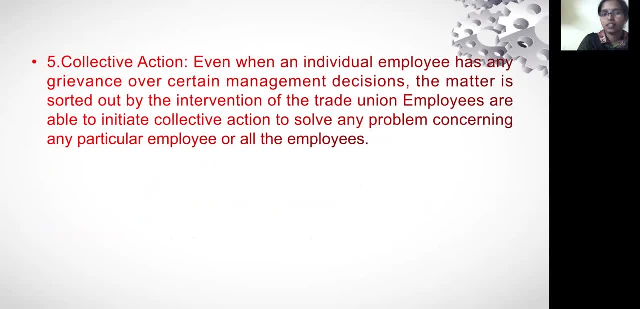 When, even when an individual have an issue with the Employee employer, The, Sorted by the intervention of trade union employers, are able to initiate collective action to solve any problem concerning to a particular person or this particular worker or Employees employer. employees are Employee, even single. if there is a problem with the management, even with the single individual or the all the workers, this the trade union will be intervening and they'll be. they'll be expressing the on behalf of all the workers. 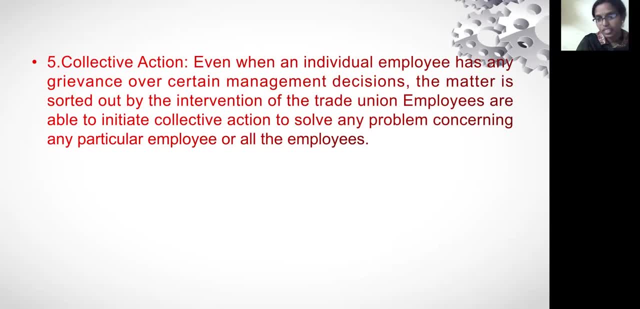 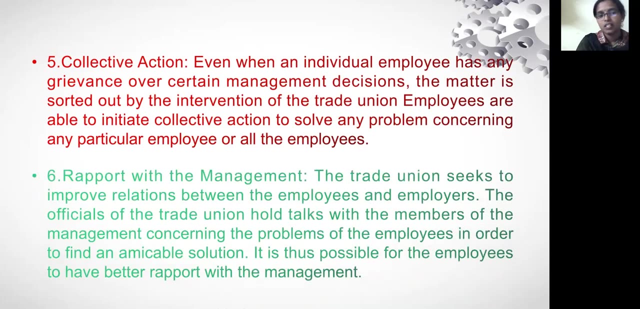 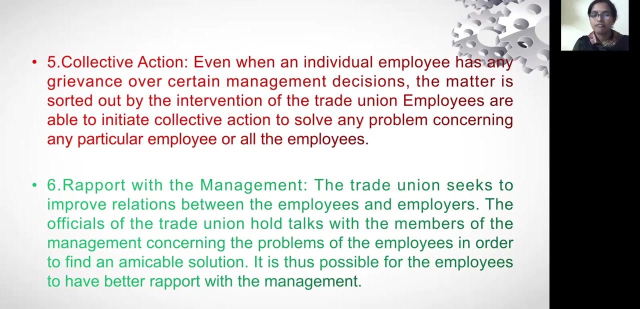 Or else on behalf of the employee employee and they'll be putting forth to the issue of the individual employee or employees before the management and try to resolve the issue with them in an amicable manner. Report with the management. the trade union seeks to improve relationship between employee and employer. the officials of the trade union hold talks with the members of the management concerning the problems. 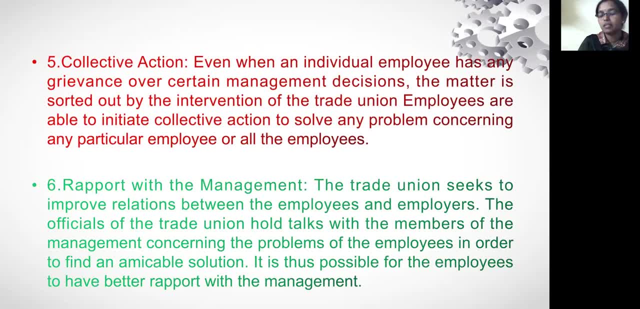 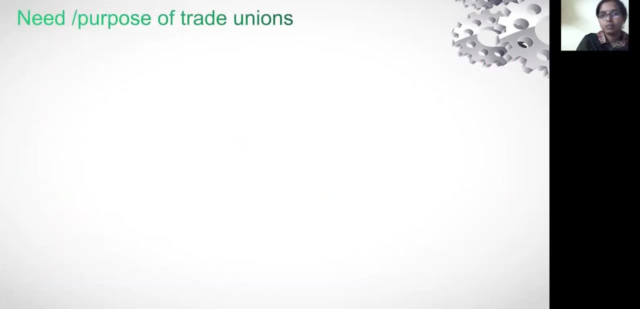 Of the employees in order to find an amicable solution. It is that's possible for the, for the this, the employer, the trade unions, to have a better rapport with the management. members of the trade union. So need and purpose of the trade union. Why we need a trade union? Why we need to join in your trade union? The purpose is for the: better wages, better working conditions, protection against exploitation. 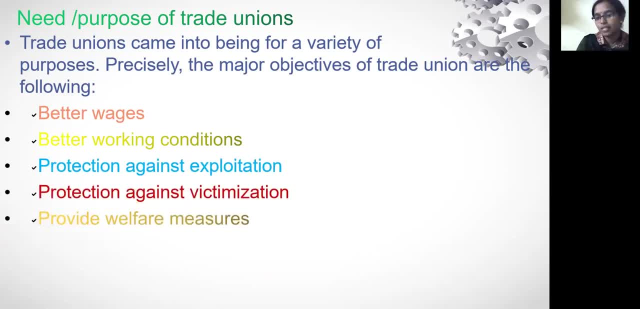 Protection against victimization. Here the victimization means beating, abusing or anything, any any illegal thing or anything That hurts the individual. So, providing welfare measures, promote industrial peace. take up collective bargaining on any regarding any issue in which involves individual employee or employees. 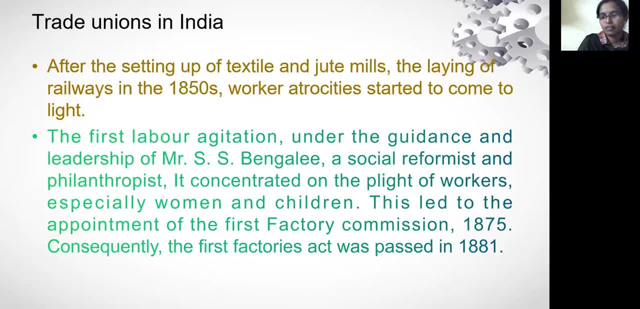 Look after the interest of the trade. These are the Main purpose why we join into the trade union. So trade union in India, So we'll be coming to the trade union is in India. So before discussing about the Advent of this trade union, will talk about a small brief of a lab moment, because the lab moment is has paid a part for the trade union moment in India. 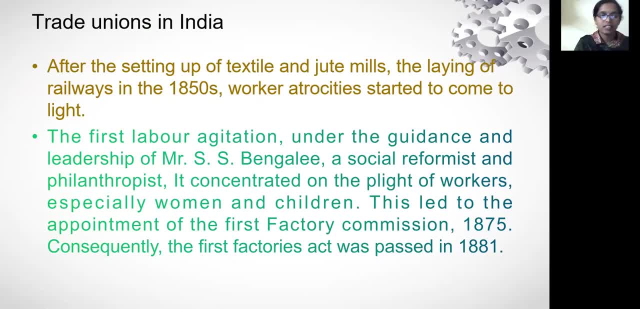 So the lab moment in India, So, as we said, which has been Started As a response to the, as a response to the unfair lab and field lab of practices of the employers in, in the, in the industries, So in the decade of 1851 to 16, which is this is a decade. 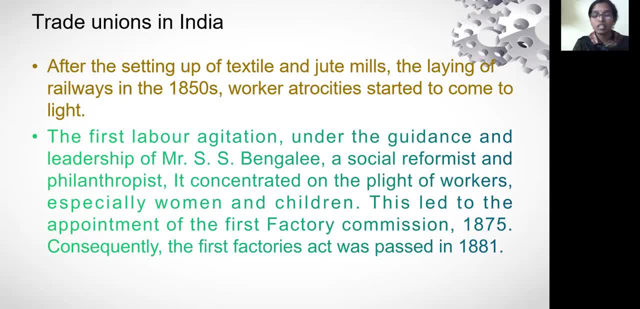 The most five sectors has been in in boom. They have started industrialized, like cotton industries, has been established in jute industries, planetation coal mines And I use these are the most important industries that came up in this decade in 1851 to 60. 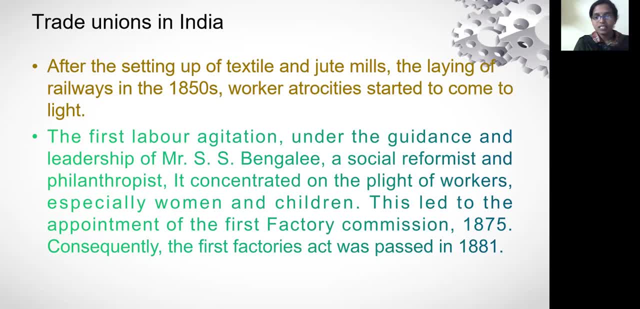 So during this time, what happened? This is a. this is the decade in which, this is a moment in which the industries came up in. industrialization took place in the country, and this Not only industrialization took place. this industrialization has been coupled with Illegal 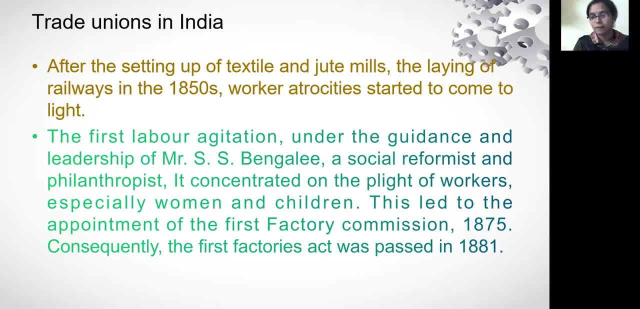 Practices, Legal Label Practices, Unfair labor practices, I can say Like low wages And slavery, and all these things to prolong the working hours, making the people to work for long hours. All this took place in at this time. So So these At this moment, after setting up the textile industry jute mills in here and laying up railways in 1951, during this decade, 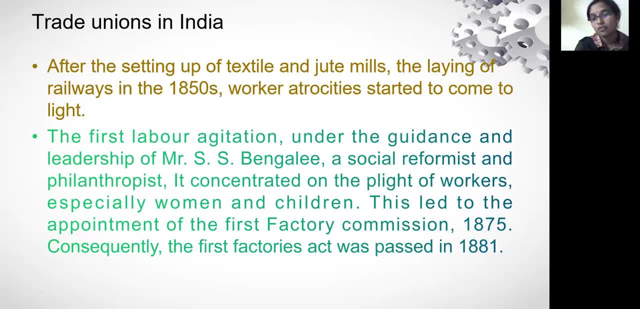 If you say 51 to 60, the worker atrocities that started to come into light. So in this industry they have, they have started a too many legislations. The British government has took up a too many legislations in this era of, in this, in this decade, like in 1951 to 60. 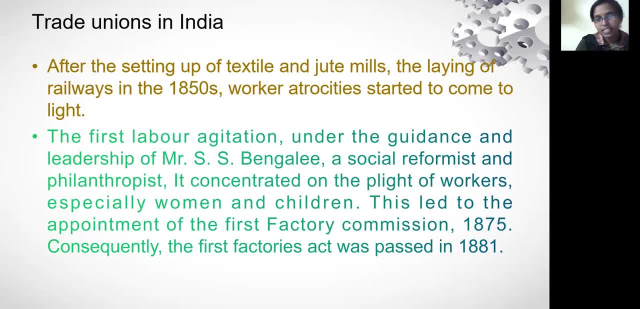 This gave rise to labo problems. to tackle these problems, What are the problems which we have discussed? Like a prolonged working hours, women and children, Putting them into manual work, maybe heavy and manual work, and to to tackle this problem The British government initiated. It is also tried to try. the British government has also tried to tackle this problem and they have initiated some of the legislations, like apprentice Apprenticeship Act of 1853 and Fatal Accidents Act of 1853. 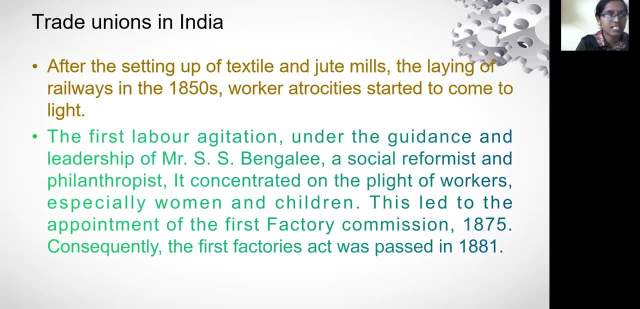 Apprenticeship Act of 1853 and Fatal Accidents Act of 1853. Apprenticeship Act of 1853 and Fatal Accidents Act of 1853 And the workers workmen beats of contract act of 1859, employers and employee and workmen disputes act of 1860.. However, all these act legislations came up by the given up by the British government, but they 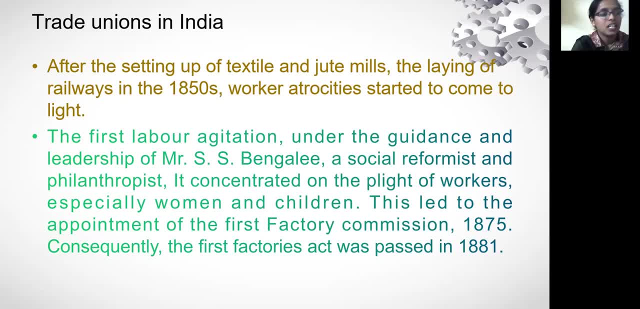 They couldn't solve the labo problem because they have been in the all this law. laws were in the interest of the employers rather than the interest of the labo. because of it, they didn't work out on the labo problem And they didn't work out to salatay. I killed the problems. all the problems have to work. lab movement in India started because of it. 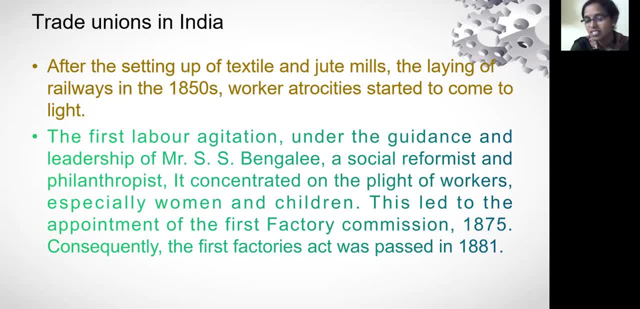 Even though the legislation in the problem doesn't solve the lab moment in India has been tough. It's the took its shape in the area of 1875. So then when this is, the British cotton mill owner met the Secretary of the State. 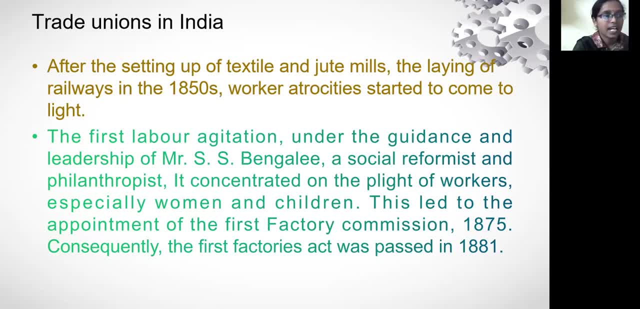 of the state for India and he has advised the government of Bombay to appoint for the appointment of a factory or an investigator, or else first of the labor commission- Bombay in this factors factories Commission, to investigate into the labor conditions. the fatal cause of this labor movement is the fear of lancashire mill owners. what the role of this? 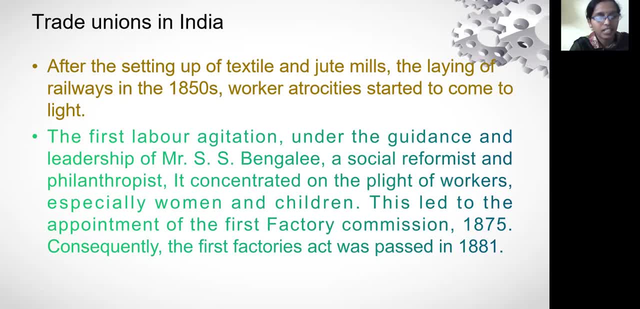 lancashire mill owners is like they used to thread the Indian sellers to sell the cloth at a very low prices. because of it, there is a biased resolution has been expressed, a resolution expressing the sorrow or against this exploitation of this mill owners by the workers of India, like 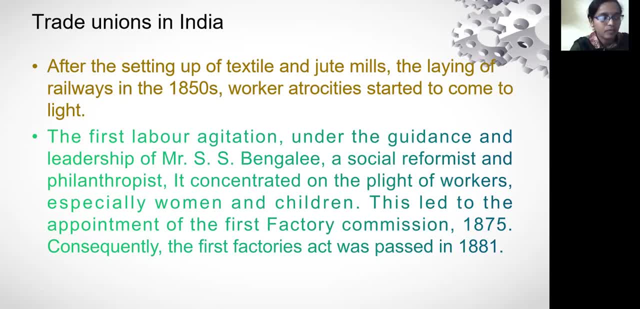 because of it, like the exploitation of female and the workers of India, like because of it, like the exploitation of female and juvenile labor in India, all this problem has been put before the British government. so they have took up a British lab first, British factors commission, Bombay factors commission has took. 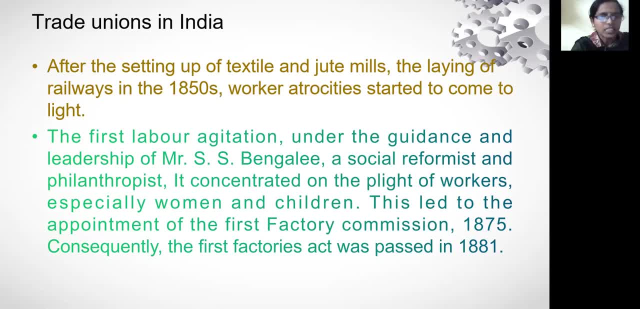 place and the first lab of hesitation, under the guidance and the leadership of Mr Yes's Bengali- he is a social reformist and a philanthropist- it concentrated on the plate of workers, especially women and children. this led to the appointment of first factory commission in the year of 1875. 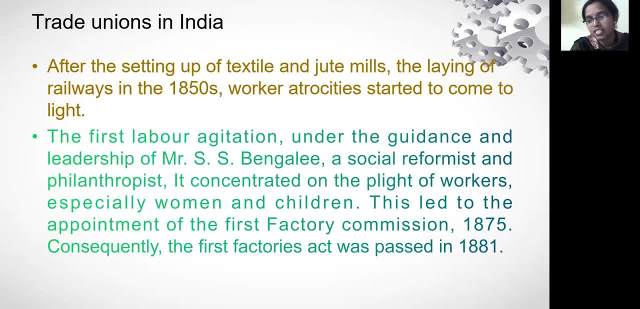 consequently, the first factories act was passed in 1881. so he is a person who has started who he's. that's why it is called as labor movement, because he's a non-worker who who hesitated for the well-being and the well-being of the people who were working for the people who were working for. 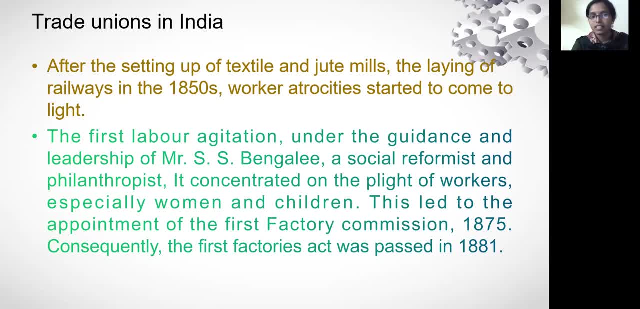 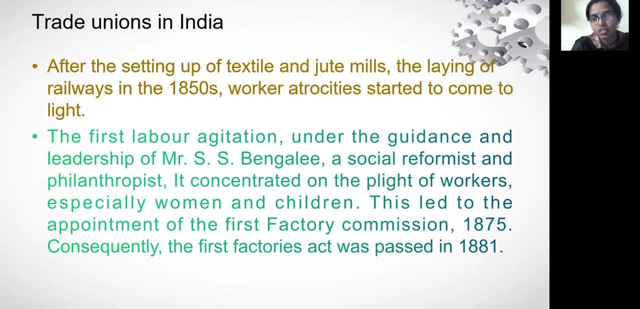 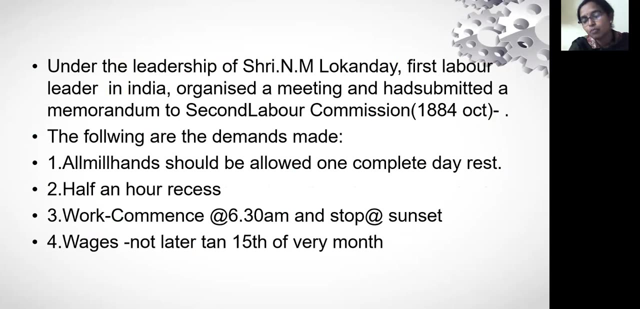 hesitation. his hesitation led to the appointment of first factory Commission in 1875 and the factory that was passed in 1881. so under the and the next under the leadership of three N M Lokhande, the first lab leaders in India organized a meeting and had submitted a momentum to the second labor for the Bommel second labor. 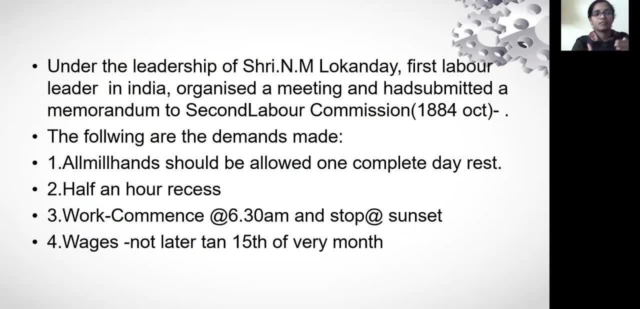 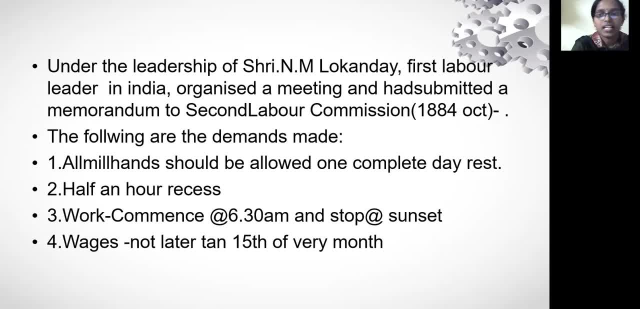 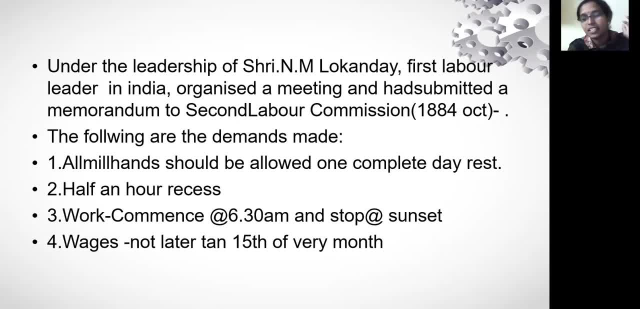 should be allowed one complete day rest, that is on Saturday. they need a one day rest and for all the workers and half an hour break during the afternoon and they have to all the workers. the work has to come in comments at 630 in the morning and has to stop at sunset and the next one is the payment of wages should be. 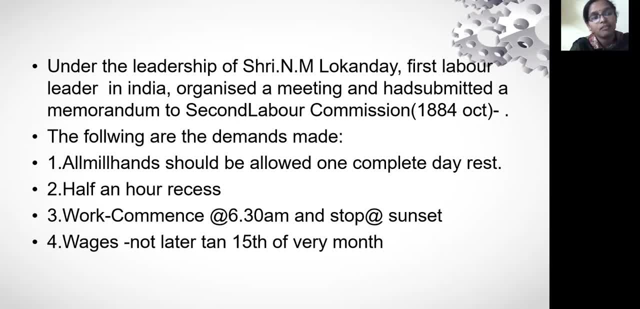 made not later than 15th of month falling for which they had been earned. and the next is women- the workmen sustaining any serious injury. and the next is women- the workmen sustaining any serious injury in the course of his work. he will be disabled because of the, because of the. 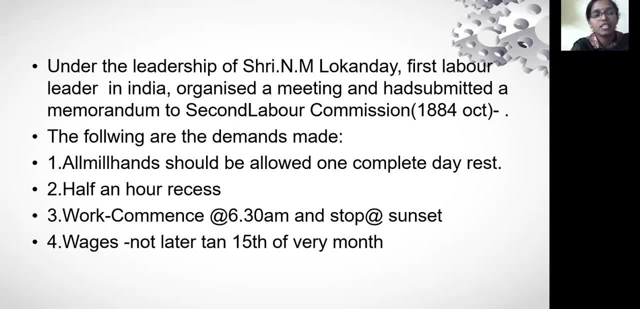 accident or something, he should receive full wage until the recovery. so these are the demands that has been put forth by the, under the leadership of C NM Lokhande, the first labor leader in in the year of 1884, October. by signing this memorandum has been signed by the first labor leader in in the year of 1884, October. by signing, this memorandum has been signed. 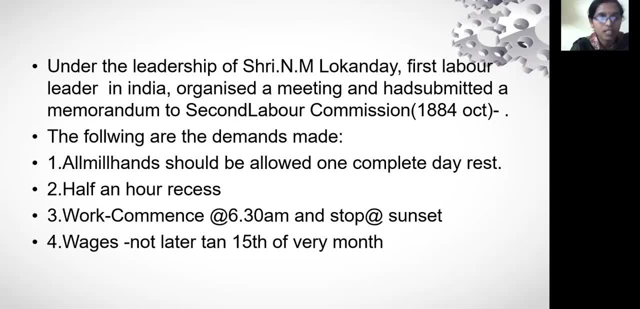 by around five thousand five hundred workers and he has given these are the following demands: one is one complete holiday, that is, on Saturday half day, like half an hour, it's not sorry, it is half an hour recess or the stoppage or the break in the afternoon. third, one is 15th of every month. they have to pay their. 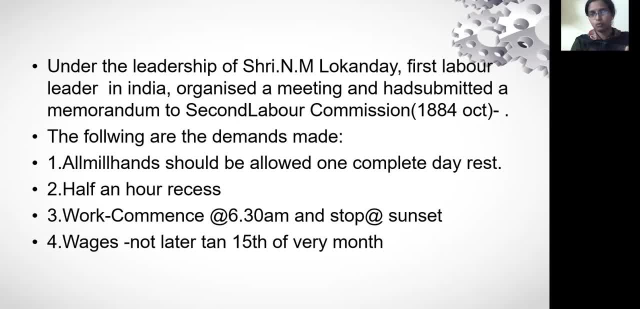 wages and work should commence every in every mill. the work should commence at 6: 30 am in the morning and should stop at sunset and the next. it is not mentioned the person who is working in the mill, if he has, if he has met with any serious injury during the course of his work and he will. 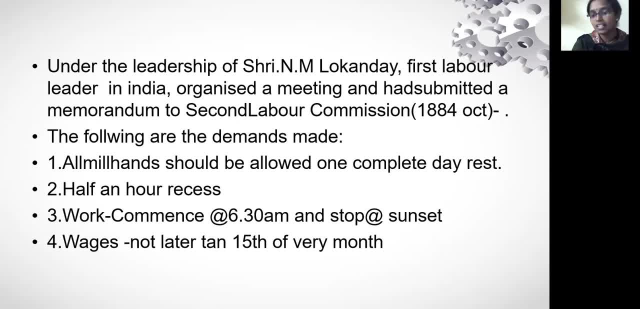 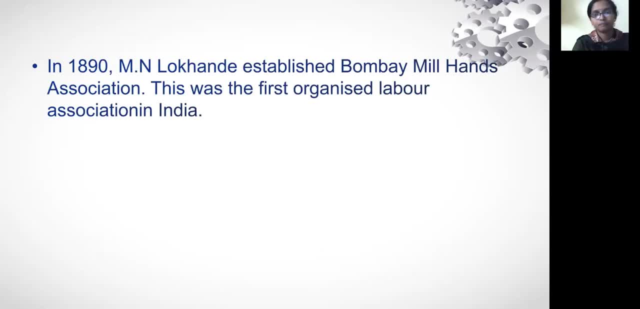 he should be. he should receive full wages until his recovery. these are the demands has been put forth and during this time and during this period of 1890 to 18- 1918, so too many association has been formed. in 1890 I mean look and established a Bombay mill hands Association. this was the 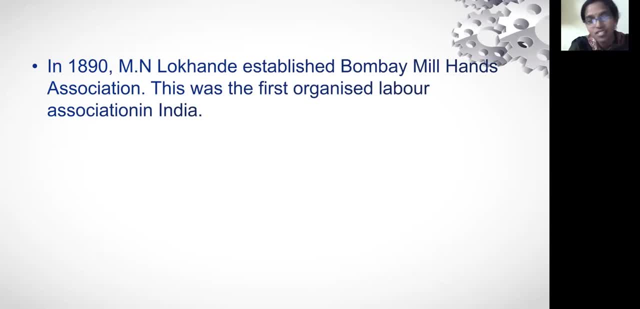 first organized labor association. this is only an association, this is not a union. and after that they have. they have. lot of associations came up, like in nine In 1897, Amalgamated Society of Railway Servants Printers Union of Calcutta in 1905, Madras and Calcutta Postal Union in 1907 were also associations formed and many more associations have been formed in the beginning of this movement. 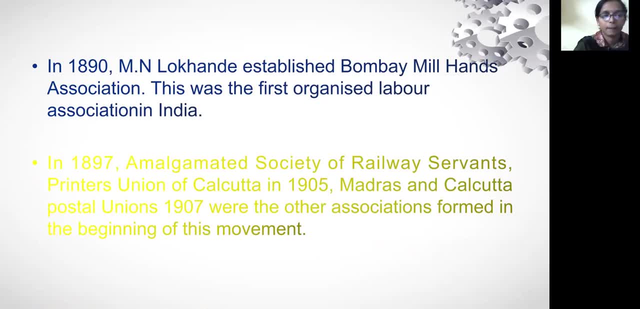 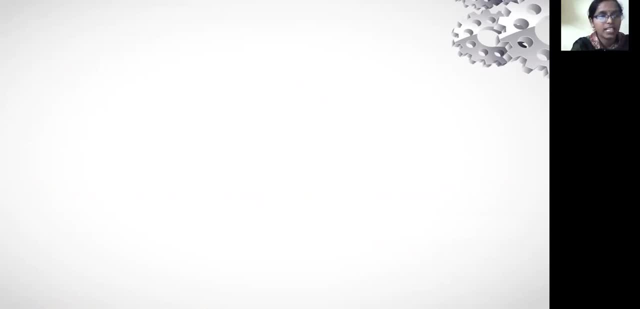 So this is how the influence, the leadership of Lokhande, has been influenced to form too many unions at that time And during this moment. this is a very important moment because 1982-1924, this is the early stage of trade union. 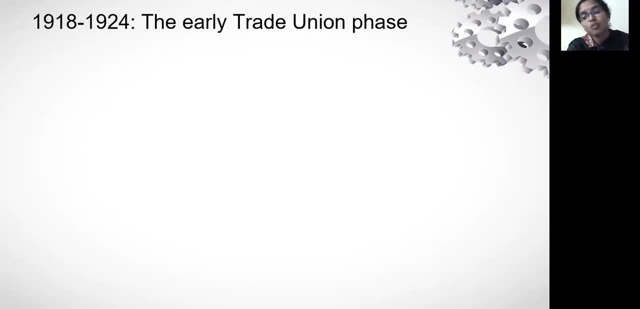 Why? Because this stage is over. This phase is also called as birth of Indian trade union movement. This stage- 1980-1924, this phase is also known as birth of Indian trade union movement. This is the early stage of the birth of trade union movement and how the trade union movement has been started. 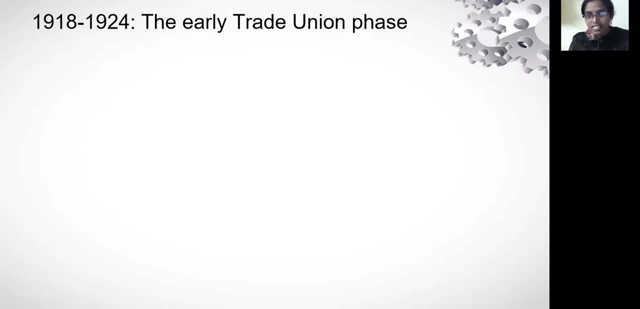 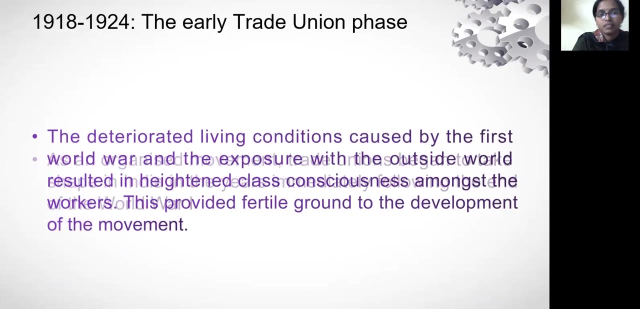 Till now we have gone through labor movement and now we are completely going through the trade union movement, How this has been After the post-war. after the war, as an organized movement, the trade unions began to took its shape in India in the years immediately following the end of the World War I. 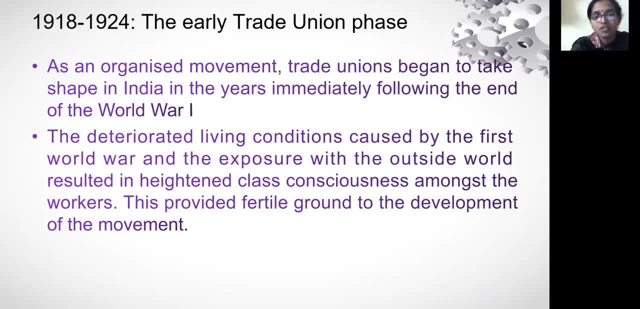 After the World War I has been commenced. the deteriorated living conditions caused by the First World War and made the people exposed to the outside world resulted in high lightning Class consciousness among the workers. This provided fertile ground to the and this provided a clear path to the development of the trade union movement. 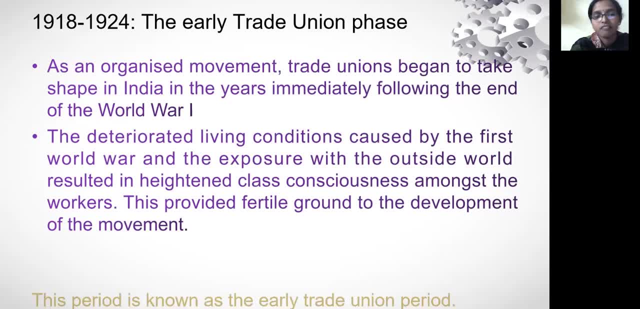 This, deteriorated working conditions and all this have made after the stroke of the World War I. this made honest think, or rethink, in the minds of the workers to form a trade union. this that's why this period is called as early trade union period. so during this, 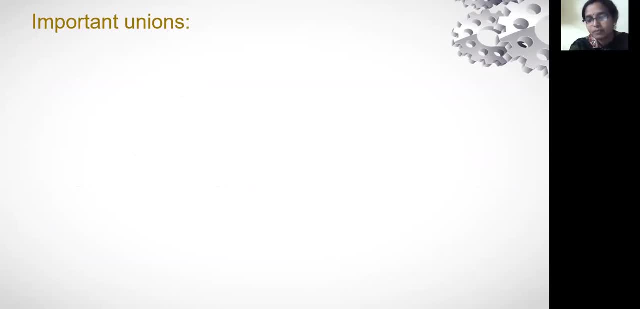 period. there are lot of things has been happened. so during this period in the year of 19th- why this period is very much in- people got very much inspired in this period and they started very, very started agitation. they are nearly in the in. from 1970 to 20 period they were nearly 30 strikes has took place in the 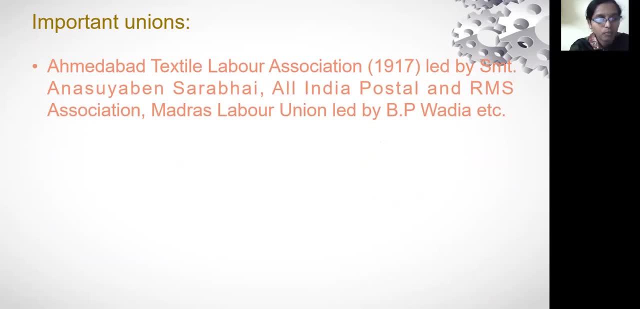 textile industries of Bombay or Amitabad, Solapur and Madras against the exploitation of the employers. so why this has happened? because in the Russian revolt in 1917 has been took place and this has led to all these wars. This has given an idea of this, has this has pointed an idea in the minds of the people. 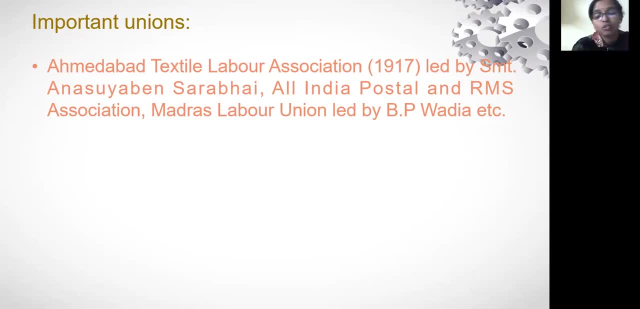 that exploitation of labor could be addressed or could be stopped by the political means. They understood that with the revolt of, with the revolt of Russia, and the Communist Party has been very much influenced with the Russian Communist Party, that I mean to say that the Communist Party of India, which has received inspiration from the USSR, captured the they. 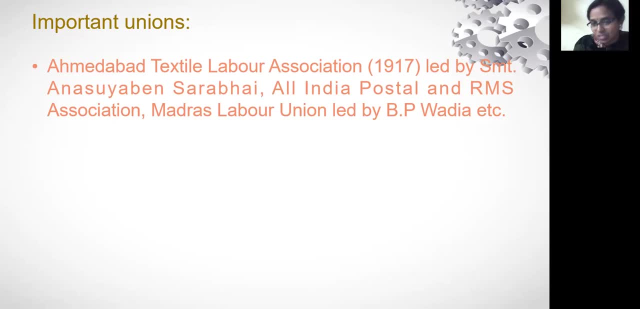 thought of forming into a union like. AITUC has been formed with the inspiration of the of Russian revolt by the Communist Party, and also the with the inspiration of ILO, International Labor Organization, which has been formed in 1919.. And this inspiration, 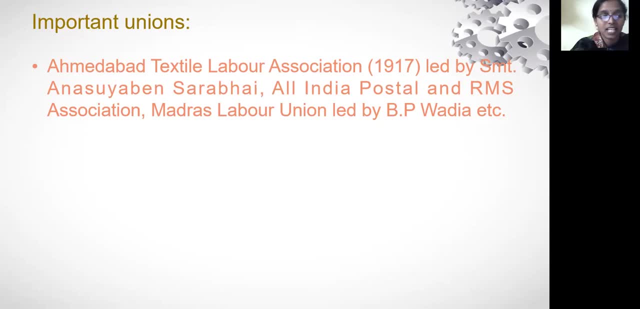 International Labor Organization, which has came into existence in 1919, it has it has which is due to Peace Treaty of Versailles in 1918. And it has- this has- profoundly influenced India's labor movement, labor legislation and labor policy. And with all these influences, like Russian revolt and 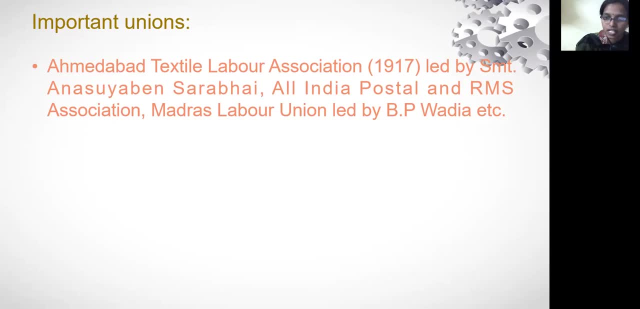 and Indian International Labor Organization. There are many trade unions have been formed trade unions. a trade association has been formed at the time, like Ahmedabad Textile Labor Association, led by Smriti Anna. So yeah, Ben Sarah, by all in your postal and RMS Association. Madras Labo union, led by BB. 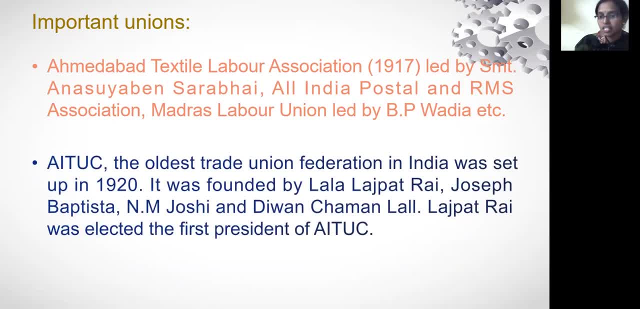 Varya. This are all various. various union came into front and AITUC has been formed. AITUC has been formed, which is one of the union. oldest trade union Federation in India was set up in the year of 1920. It was founded by Lala Lajpatrai Joseph. 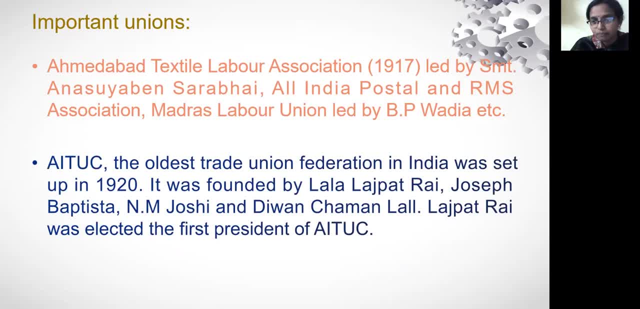 Bhattesh, NM Joshi and Diwan Chamanlal and he, Lala Lajpatrai, was elected as its president. So this is all the inspiration of the. everybody got inspired with the Russian movement, Russian revolt and ILO, which has profoundly influenced. 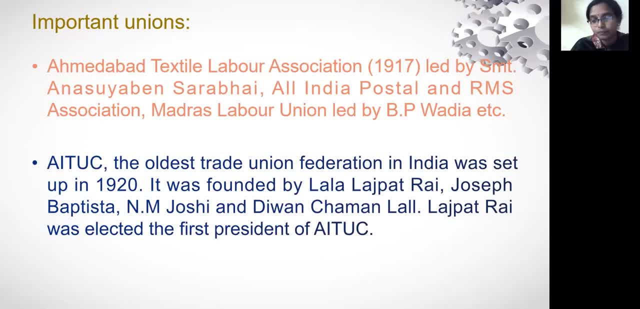 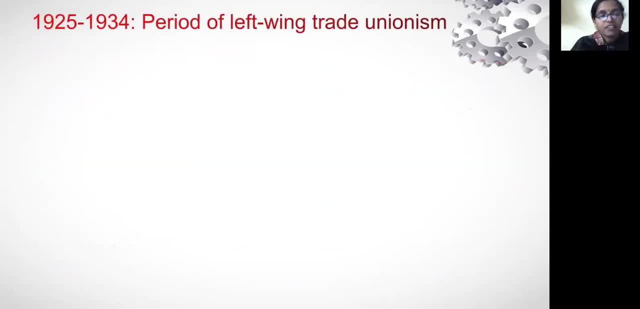 India's Labour Movement. Now we will go through the phase of 1925 to 1934. So I want to re-collect one more. in one more incident that has infiltrator the trade union was violence andعدumer allotment точка. 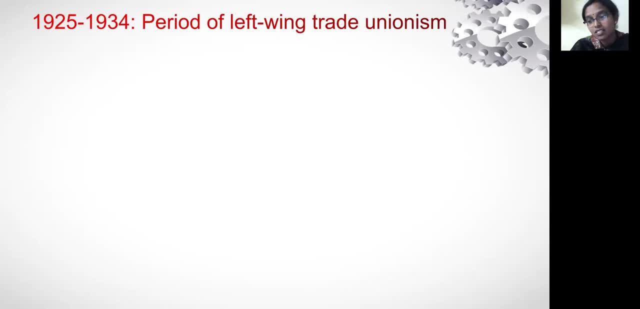 ン movement is. I can remember, in 1920, August. in the month of August, Mahatma Gandhi's first civil obedience movement started. This civil obedience movement has also added some wings and some feathers to this trade union movement in India. Why? Because it has provided too many young. 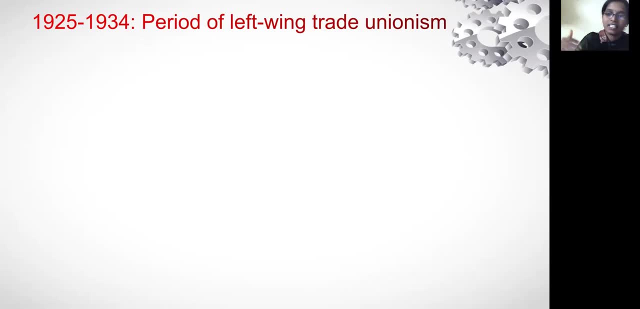 energetic and dedicated and inexperienced leaders to the trade union. Too many people have come out of their shelves with a lot of passion, energy and they have introduced it to the trade union movement with the civil disobedience movement in the year of 1920. So this all has impacted the trade union movement. 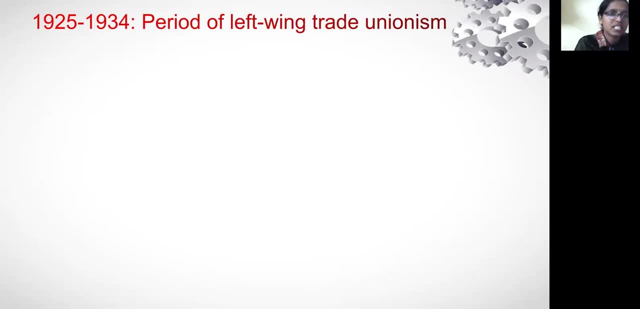 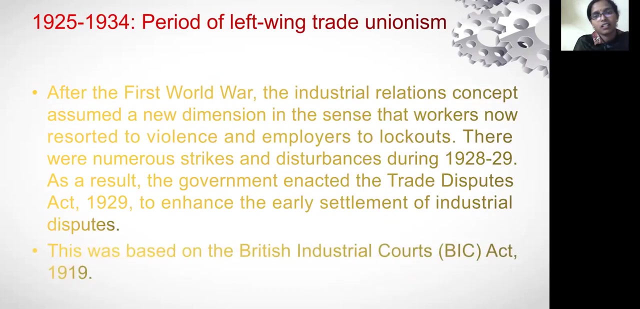 for the birth of the trade union movement and coming to the next phase in 1925 to 1934,. this moment, this phase, is called the period of left wing trade unionism. So after the first world war, the industrial relations concept assumed a new dimension in 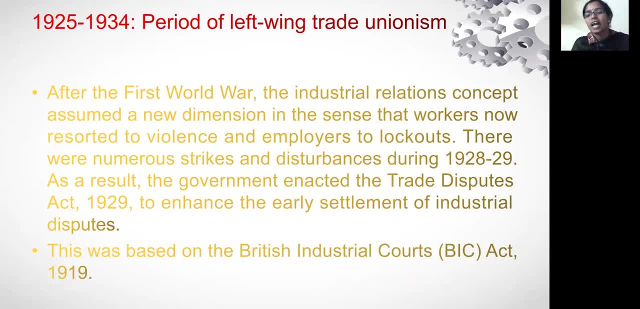 the sense that workers now restore to violence and employees to lockdown. There were numerous strikes and disturbances during the 1928 to 29.. As a result, the government enacted the Trade Discrude Act of 1929, To enhance the early settlement of industrial dispute. this was based on the British Industrial 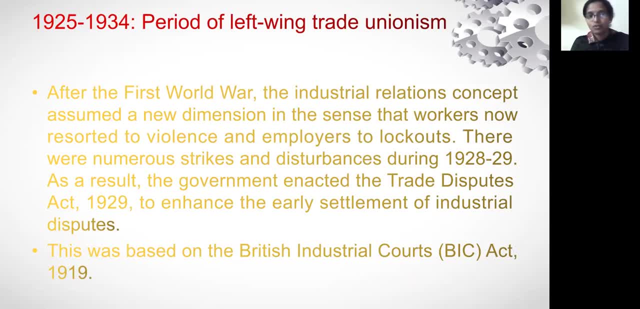 Code, the BIC Act of 1919.. So in this period, 1928 to 1929, there were an enormous number of strikes and disturbances, in industrial unrest that took place and, from the employer point of view, they have started lockdowns. 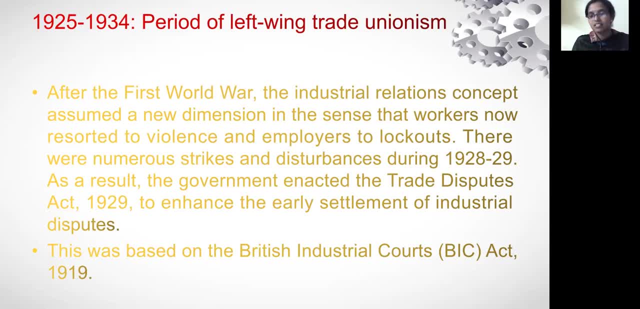 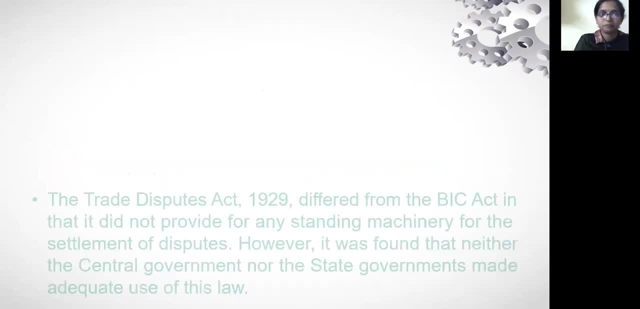 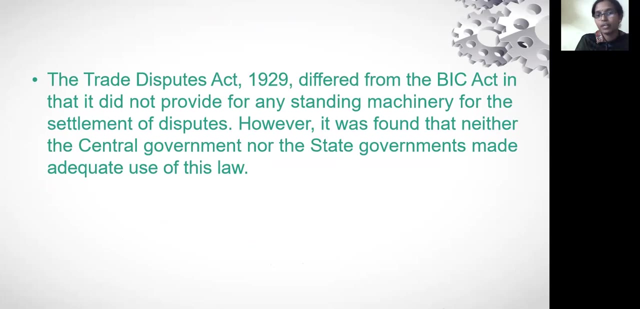 So, because of all these disturbances, the government enacted Trade Dispute Act of 1929 for the control of all these disturbances, industrial unrest. The Trade Unions Act of 1929 differed from BIC in it did not provide for any standing missionary for the settlement of disputes. 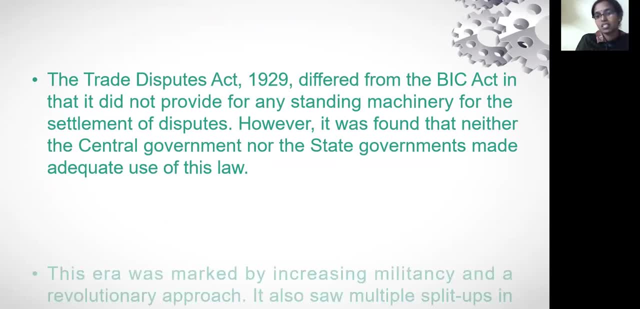 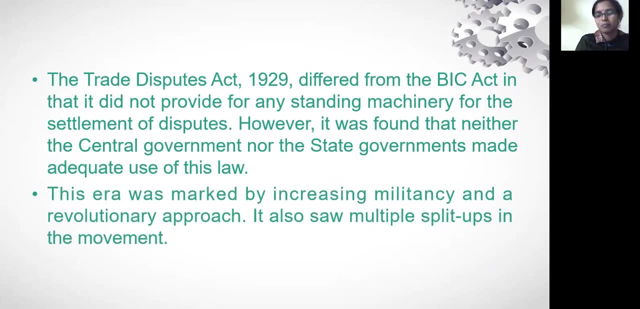 So, however, it was found that neither the central government nor the state government made the adequate use of this law. So in this era, this was marked Militancy, militancy like agitation and the revolutionary approach. everybody has become very revolutionary, all the labours has become very revolutionary and energetic. okay, and 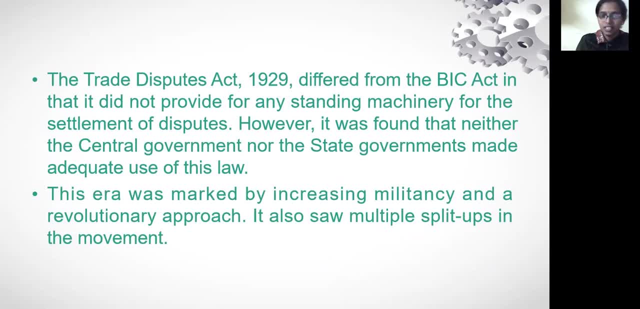 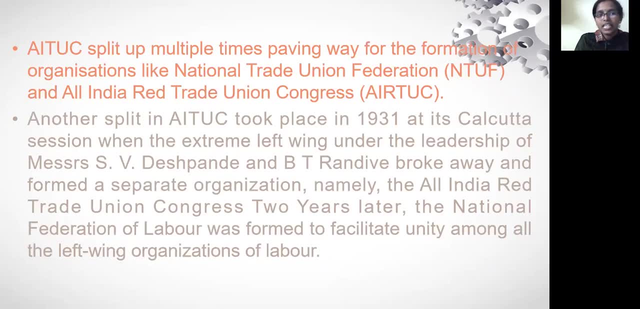 they are into a mood of revolution, revolt against the unlawful practices. It also saw multiple split of the movement. At this time, AI to use this split up multiple times. They are being paid for the formation of various organisations like National Trade Union Federation, NTUF, and All India Red Trade Union Congress, AIRTUC. 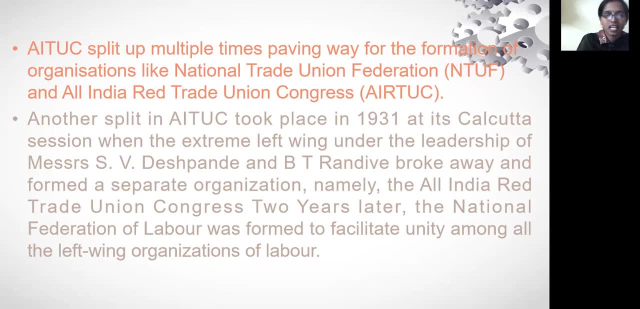 The trade union has been formed in 1920 and in this in after that, from 1925 to 34, around. there is a lot of split in this union. and another split, AIRTUC, took place in 1931. At this Calcutta session, when the extreme left wing, under the leadership of Deshpande and 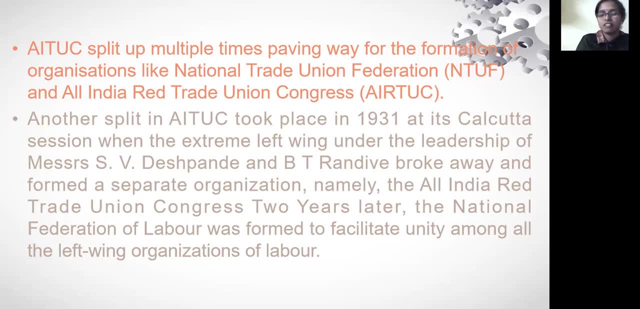 BT Dunwane broke away and broke away from the AIRTUC, and they have formed into separate unions which we have discussed, like All India Red Trade Union Congress, and two years later the National Federation of Labours was also formed to facilitate unity among all the left wing. 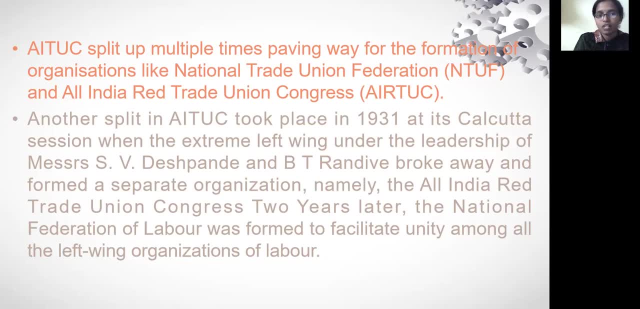 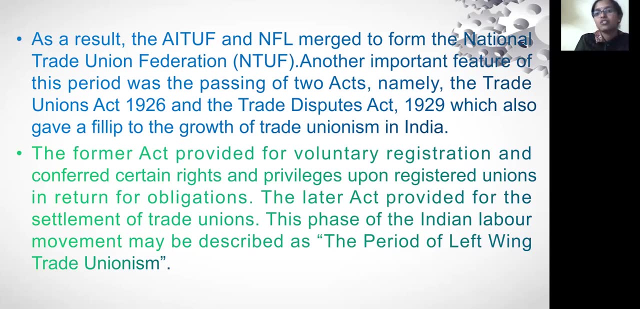 organisations of the labours. So, as a result, the AIRTUC, AIRTUF and NFL merged to the National Trade Union Federation. They have merged into this the ATUF. another important feature of this period was the passing of two acts. 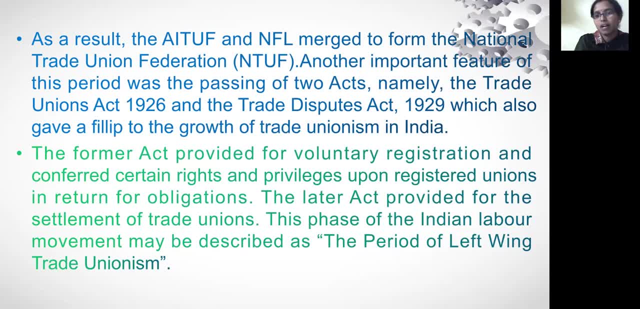 And during this period two acts has been passed. One is Trade Unions Act of 1926 and the Trade Dispute Act of 1929, which also gave a fillet to the trade union. So this is the trade union act of 1926 and the trade dispute act of 1929, which also 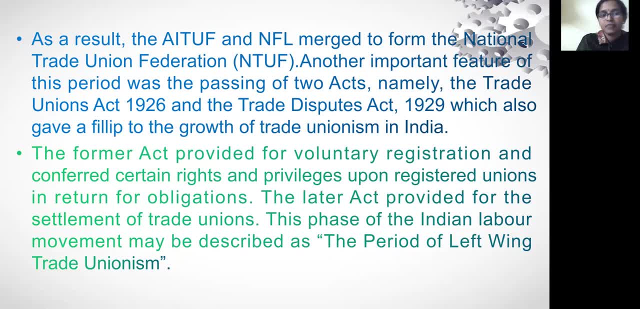 gave a fillet to the growth of the trade unionism in India. The former act provided- and that is the former act means the first one- the Trade Unions Act of 1926 has it is voluntary registration of the trade union. okay. 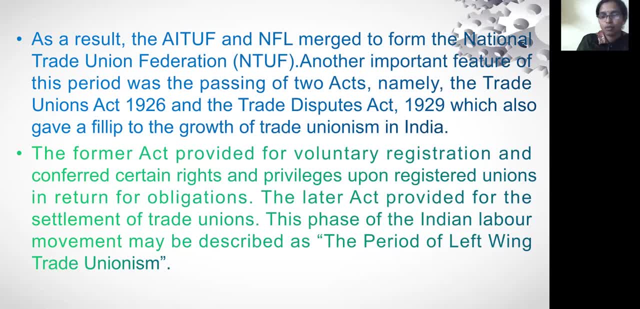 It has formed from provisions for the registration and provisions in the process for the registration of trade unions. So and later is the dispute act of 1929. So this is the trade union act of 1929. So this is the trade union act of 1929. 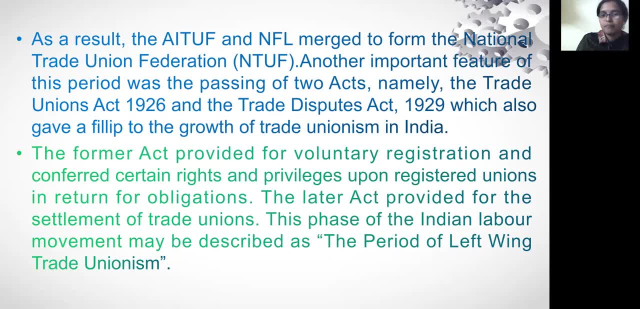 So this is the trade union act of 1929.. So this is one the later provided for the settlement of trade unions. So this is the trade union act of 1929.. So this is the Trade Unions Act of 1929.. 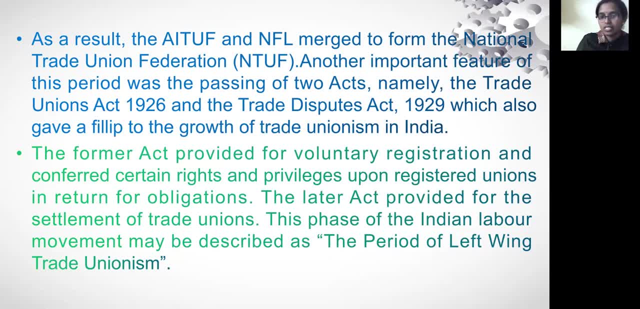 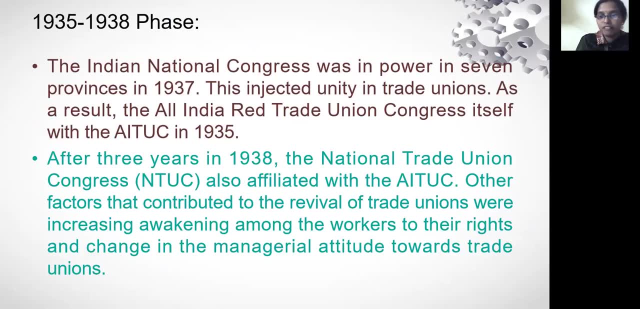 This was declared the trade dispute act of 1920.. The trade dispute act of 1931, this latter provided for the settlement of trade union. in this phase of trade union, labor movement was described up period of left-wing trade union and during this left-wing trade union there is lot of partitions of fragmentation has 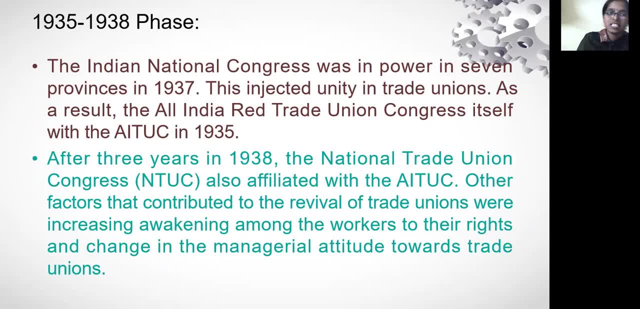 been taken to place during this period. In 1935 to 1938 phase, the Indian National Congress was formed and eight national fairly was in power in even seven provisions of 1937. This injected unity in the unions Again. the split trade unions has been again reunited at the next stage. 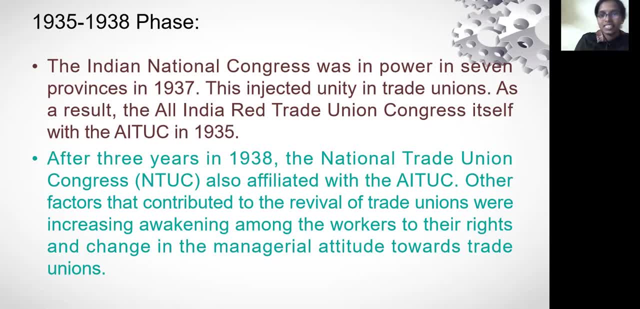 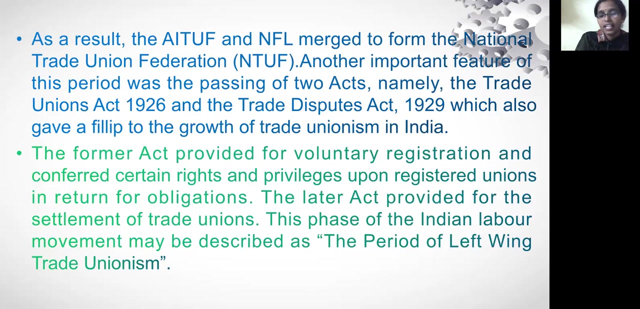 like at this stage of 1935 to 1938.. As a result, the All India Red Trade Union Congress itself with the AITUC in 1935.. In the before stage they have split into two different unions: One is the All India Red Trade Union and the ANFU and the NFL. and now, in the next stage, 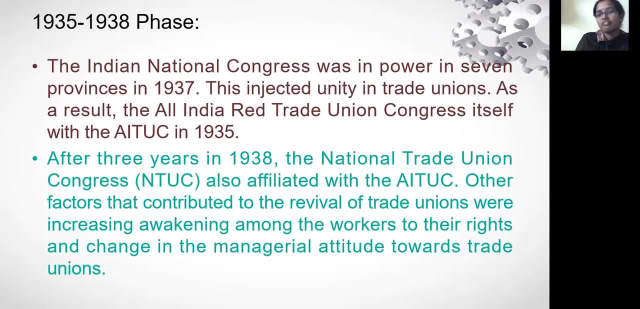 they have reunited into AITUC After three years. in 1938, the National Trade Union Congress, NTUC, also affiliated with AITUC. Other factors that contributed to the revival of trade unions were increasing awakenings among the world. In 1935, the National Trade Union Congress- NTUC. also affiliated with AITUC. Other factors that contributed to the revival of trade unions were increasing awakenings among the world. In 1935, the National Trade Union Congress, NTUC, also affiliated with AITUC. Other factors that contributed to the revival of trade unions were: increasing awakenings among the world. In 1935, the National Trade Union Congress, NTUC, also affiliated with AITUC. Other factors that contributed to the revival of trade unions were increasing awakenings among the world. In 1935, the National Trade Union Congress, NTUC. also affiliated with AITUC. Other factors that contributed to the revival of trade unions were increasing awakenings among the world. In 1935, the National Trade Union Congress, NTUC, also affiliated with AITUC. Other factors that contributed to the revival of trade unions were: 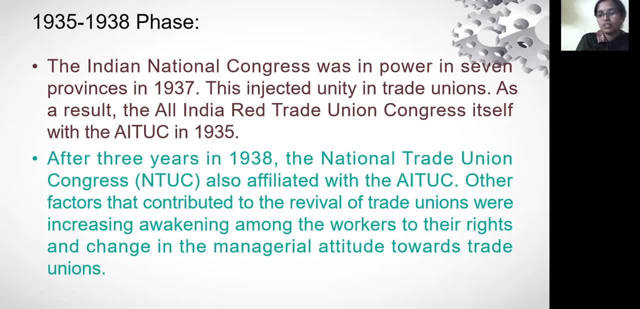 increasing awakenings among the world. In 1935, the National Trade Union Congress, NTUC, also affiliated with AITUC. Other factors that contributed to the revival of trade unions were this: why they have again reunited: means to bring to strengthen themselves. and there is also a 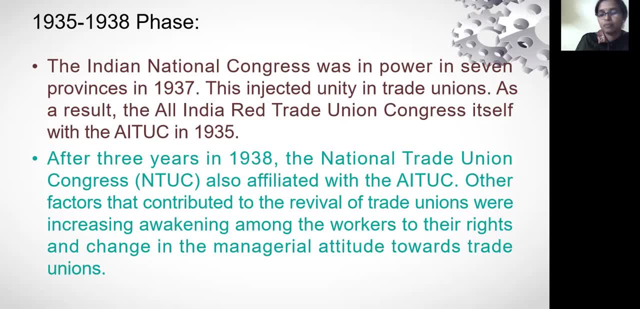 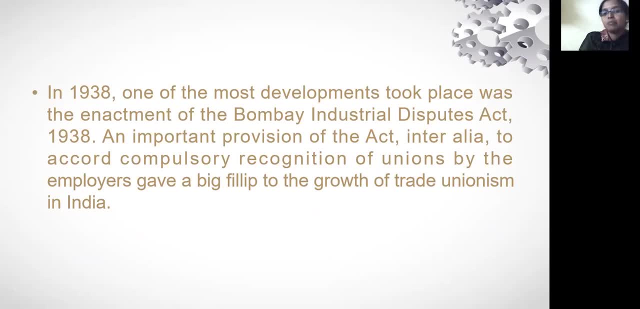 change in the minds, of the managerial attitude because of they have again reunited. and in the year of 1938 one of the most development took place was enactment of bombay industrial dispute act of 1938.. this is an important provision of the act. to compulsory it is, it is to accord to. 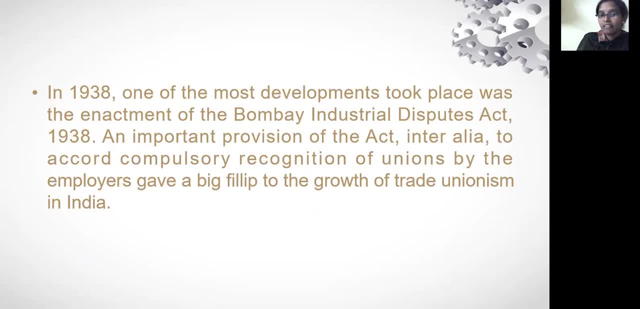 compulsory recognition of unions by the employers gave a big flip to the growth of trade unionism in india. so it has it has. it is the bombay industrial dispute act of 1930 and has has given a lot of importance recognition to the trade unionism in india for the growth of trade unionism in a 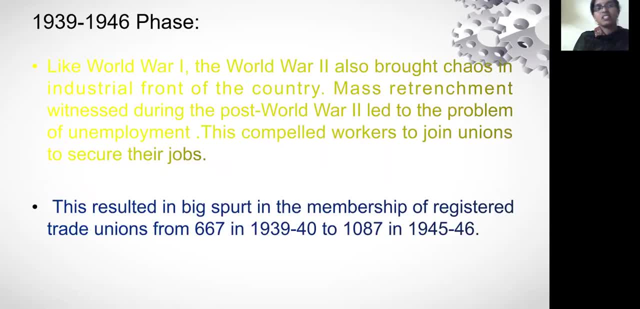 country. so in next stage of uh trade union movement is 1939 to 1946. in this phase this is our. like world war one, the broke of world war ii also brought chaos in the lot of difficulties and deterioration, deteriorative conditions in the industrial front from the country. so 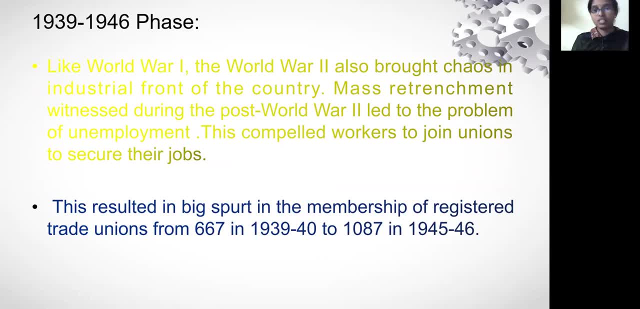 and there is a mass retrenchment to the witness. during the post world war ii, this led to the problem of unemployment. lot of people has been terminated from their jobs. this has been led to the led to the lot of unemployment and starvation and a lot of industrial unemployment. 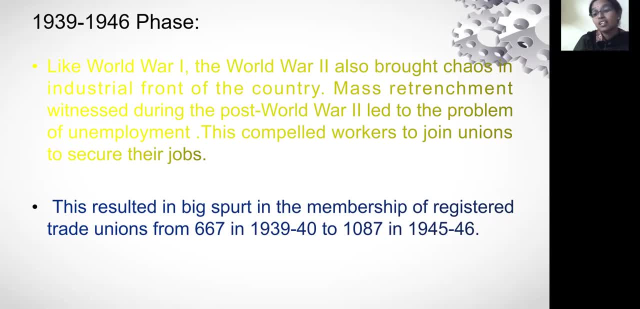 these compelled workers to join into unions in order to secure their jobs. this resulted in the big spurge they. because of this, because of the deteriorative conditions that has been revealed after the broke of the world war ii, the people joined. the people started joining into or took a membership into trade unions. they have registered. number of registered. 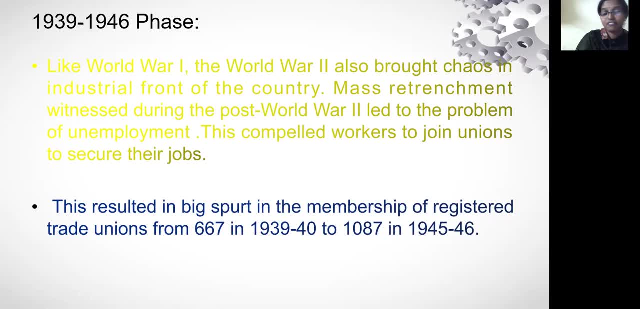 trade units has been increased from 667 to 1.3 million people in the world in the last six to six in 1939 to 1,087 in 1945. There is a drastic increase in the number of registered trade unions in the country. 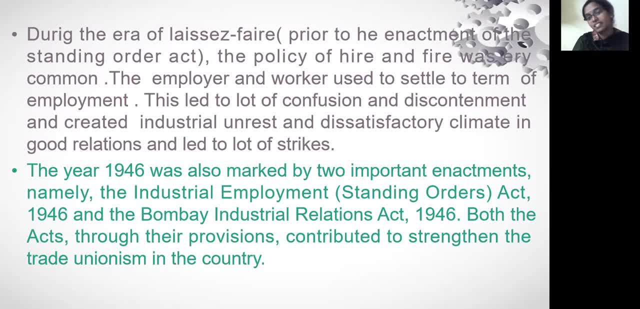 During the era of LESA 5, so before the standing order act, before this trade unionism or labor movement at the time of pre-independence. I can say that before this what happened? this LESA 5 policy has been, most probably has been followed by the employers. 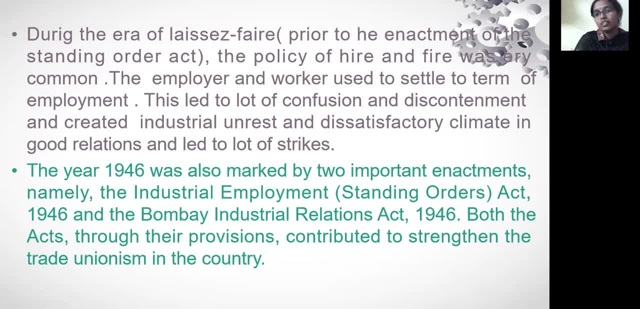 So, during the era of LESA 5, prior this enactment of this standing order act, this policy, this LESA 5, is nothing but hair and fire policy. It is nothing but the policy of hair and fire- there was a common policy that has been followed. 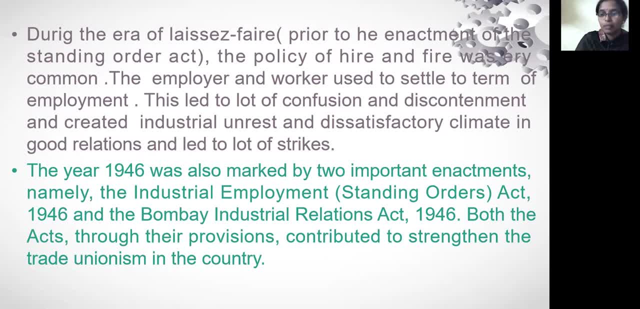 by the employer during that pre-liberalization, globalization era, pre-globalization and liberalization era. So during that era the people- the employer and worker- used to settle a term of employment, They used to have a contract, they used to sign a contract. 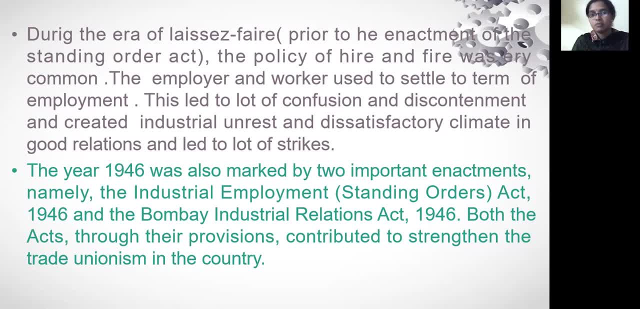 they used to have a contractual terms between the employee. either it can be implicitly or explicitly, it can be implicitly or explicitly, it can be implicitly or explicitly. they used to have a contract between the employer and employer And whenever there is a need for the workmen. 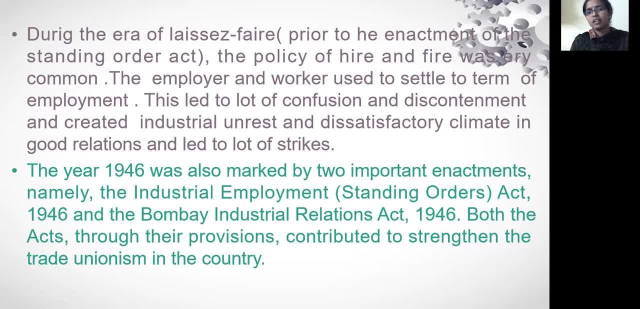 the employer used to have recruitment, or else they used to hire the people for the production purpose, And whenever the work is done they used to fire the employees. This has made a lot of confusion and discontentment and a lot of industrial unrest, And this satisfactory climate has been created. 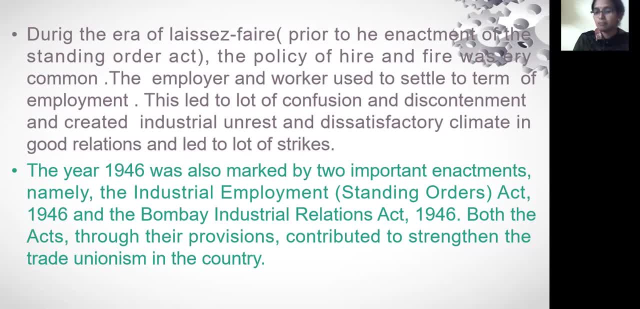 in the industry, in the minds of the employees So, and this had deteriorated the good relations and led to the lot of strikes in the industries. So, because of this, hair and fire policy, hair and fire policy. hair and fire policy. 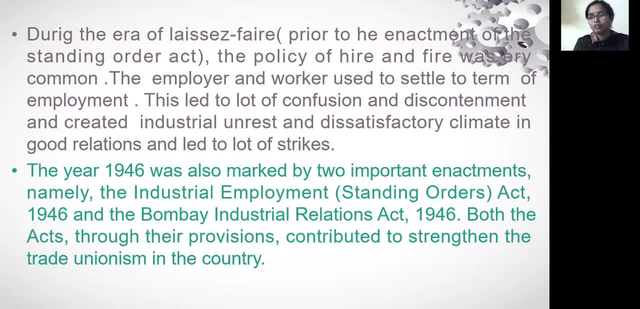 whenever there is a need, they used to hire the people whenever they have done with the because the hair and fire policies. it depends upon the supply and demand. Whenever there is a production need, they used to hire the people. whenever there is no demand. 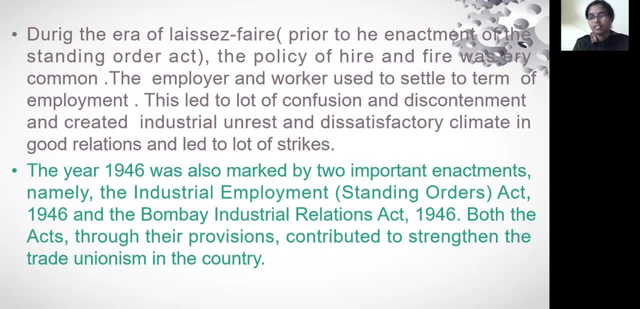 or no production. they used to fire the employees, and the employees are left unemployed. The workers are left unemployed, So because of it, the lot of strike has been took. the year of 1946 was also marked by two important enactments. 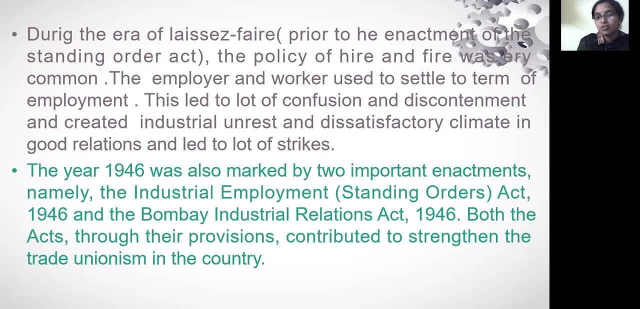 One is the industrial employment. Why? Because there is no standing orders. There is no standing orders for the employment. So because of this, in 1946, the Industrial Employment Act has been came into force and the Bombay Industrial Relations Act of 1946. 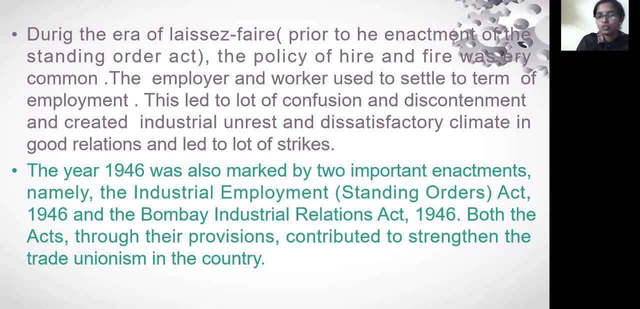 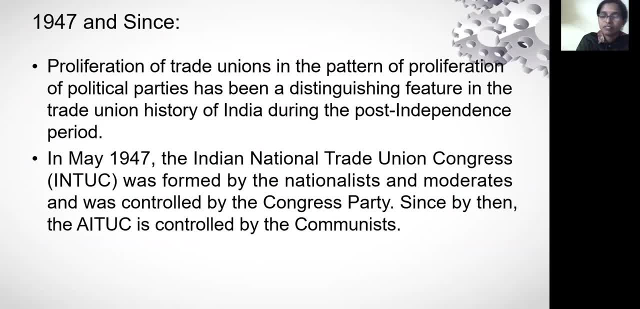 Also contributed to strengthen the trade unionism in the country After 19,Ç, since 1947 and since there are a lot of political parties influenced by post independence, the trade union on the trade unions has been a loud, a lot of influence of the political parties. 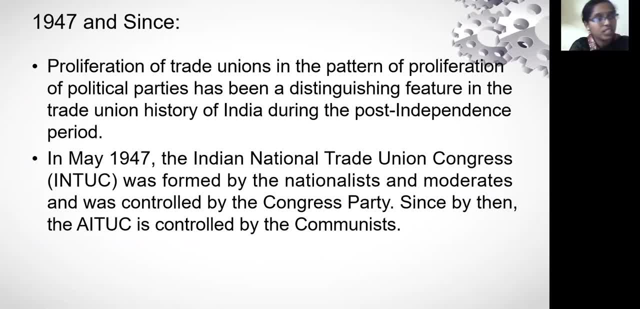 has been on the trade unions. a lot of influence of the political parties has been on the trade unions. So there is a lot of political influence. So there is a lot of political influence, okay, the labo. so the trade unions are increasingly preoccupied with the political issues. so political, 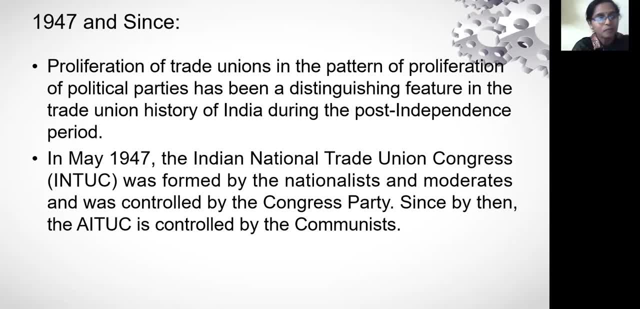 issues rather than the industrial and economic matters, and they become inherently weak and they have low membership and uncertain finances because of their weak bargaining power and relay increasingly on the legislative provisions. so, and after the independence that too many trade unions have been formed and all these trade unions have been has been increasingly preoccupied with. 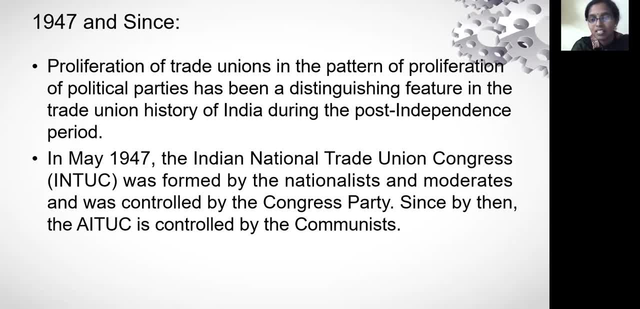 the political political parties, or it has been. they have lot of political influences on the trade unions. in 19 in may 1947, the indian trade union intuc has been formed by the nationalists and the moderates and was controlled by the congress party. since then, ait use is controlled. 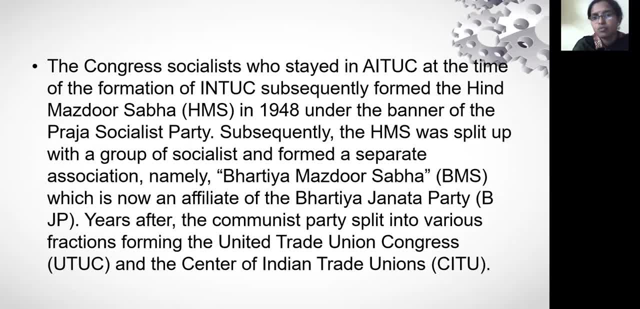 by the, the, the AITUC at the time of formation of intuc formed. so during AITUC at the time, the people who has the AITUC has been generally. the AITUC has been, has been mostly controlled by a communist and the, so the congress socialists. 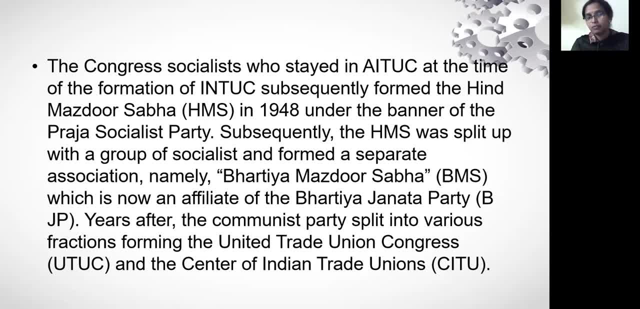 who has stayed in AITUC has been in at the time in during the formation of intuc- has been mostly controlled by a communist and the. so the congress socialists, who has been in at the time in during the formation of intuc, has been mostly controlled by a communist and the. so the 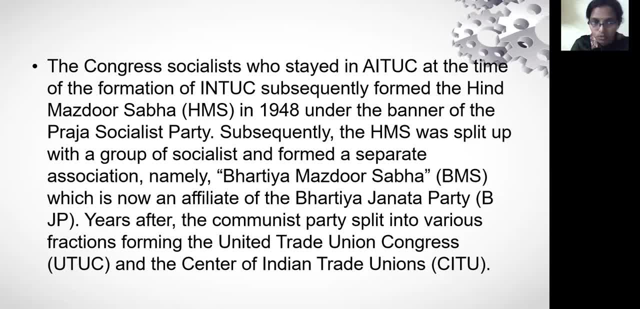 so the congress socialists were the people who have been in at the time in during the formation of intuc bans s of the union, and they have become into use. subsequently they have formed into another group, like hint masjood Saba in 1948, under the banner of a 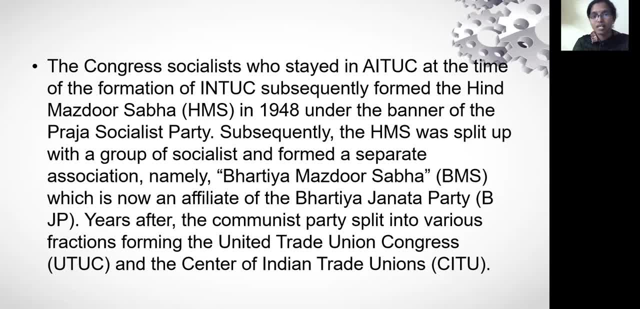 under the banner of a praja Socialist party. subsequently, HSS was split up with the group of socialists and again it has been separated, is formed into a separate association like BMS bharatiya, janatha bharatiya, masjood Saba. 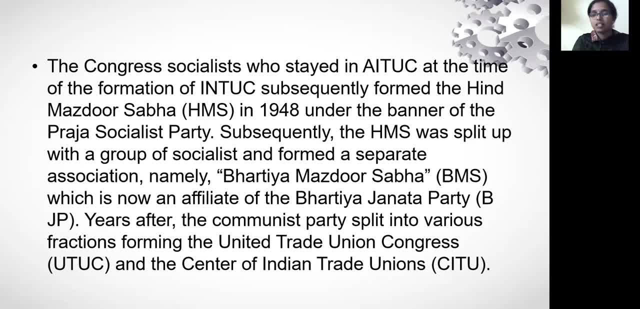 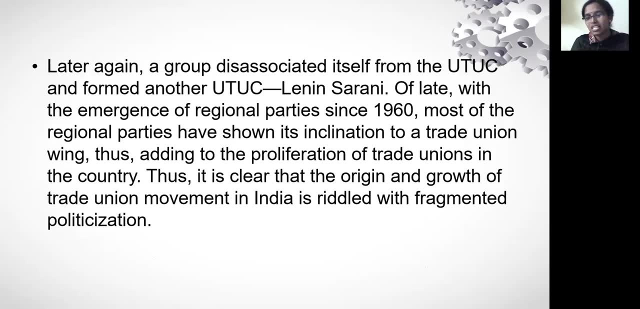 which is now affiliated to bharatiya janatha party BJP. years later, the Communist Party split into various fractions, forming United Trade Union Congress and the Central Trade Union, CITU. Later, again, this means there is lot of fragmentation has been in took place because of the, because the unions has been riddled with fragmented. 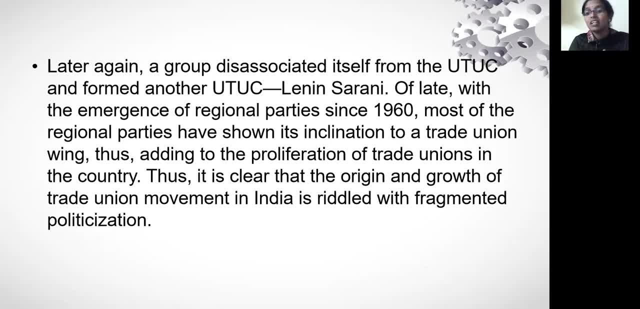 politicization. Political parties has been influenced. the trade unions has been influenced by the political party. lot of political influence has been took place in took place in the trade unions. because of it, a lot of fragmentation has been took place in the trade union. Later again, a group 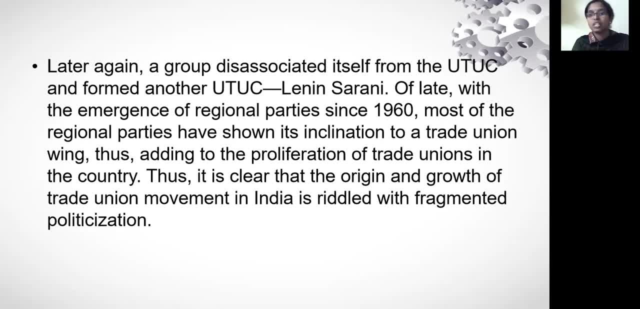 disassociation itself from the UTUC and formed another UTUC- Lenin Sarani. of late, with the emergence of regional parties since 1916, most of the regional parties has shown its inclination to trade union wing, thus adding prolification of trade unions in the country. Thus it is very clear that 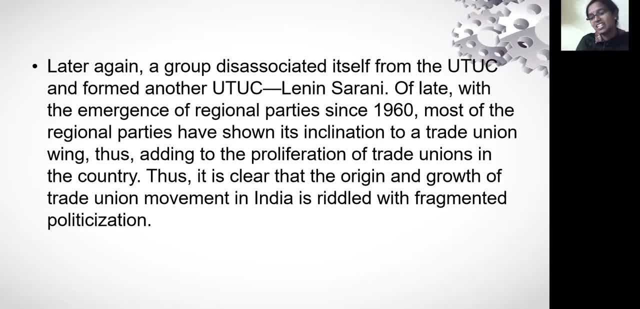 origin and the growth of trade union movement in India is riddled with the fragmented politicization. It is very clear that because of it, because of as the trade unions are increasing, because the trade unions are increasingly preoccupied with the political issues rather than with the industrial and economic matters, 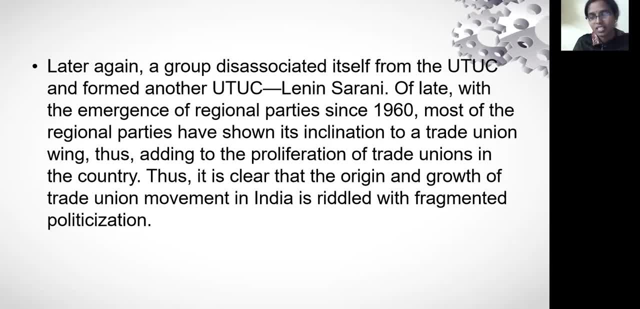 they become inherently weak Day to day. they are becoming inherently weak and compounded with their weak bargaining power and anducks they have low membership and unswept finance them. and they have low membership and unswept fine isses because of the weak bargaining power and really they most. 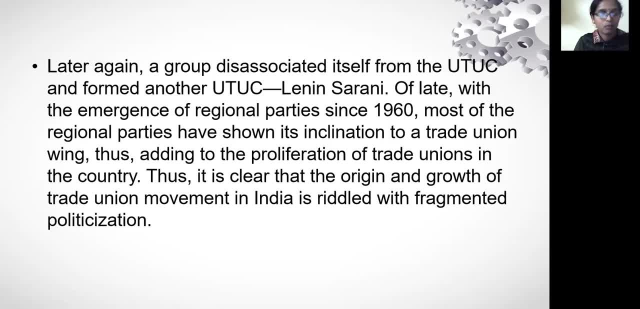 probably they use to really increasing long legislative margins and not not on bargaining power. So a political unionism, divided, divides the movement on political lines and increases Rivalry. So the political- what if trade unions is influenced by the Political parties? What happens season? 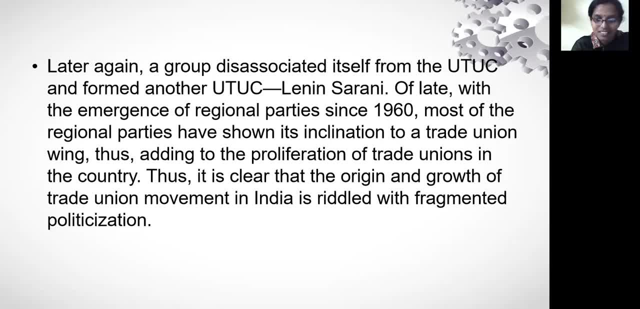 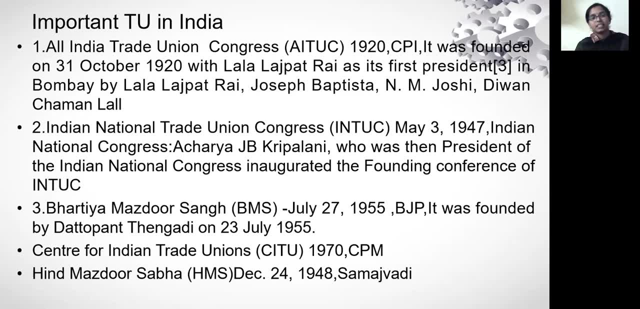 divides the movement on political lines and they develop rivalries. So these are the some of the important trade unions in India. AITUC and the political party is also mentioned there- All India Trade Union Congress, AITUC, established in the year of 1920.. 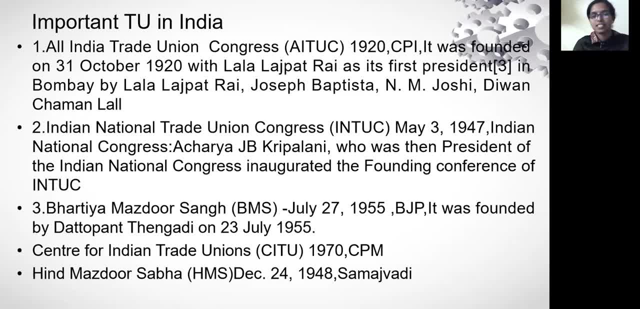 It was founded on 31st of October 1920 with Lala Lajpatra as its president And the other members Joshi Barthesh and Anum Joshi. INTUC- Indian National Trade Union Congress- formed in the year of 1947, May 3rd, and Acharya JB Kripalani was the president of INTUC. 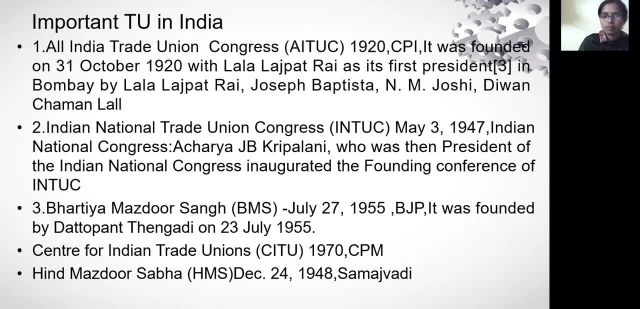 And BMS Bharatiya Masjid Sangh has been passed, formed in the year of 1955, July 27th, and in the year of 1955.. Bhattopanth Dattopanth Dengadi on 23rd July 1955. 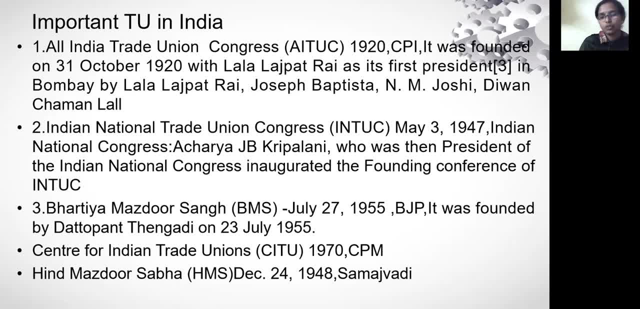 Centre for Indian Trade Union, CITU, has been formed in the year of 1917.. And the political party CPM is the. it is influenced by CPM And HMS Hind Masjid Sabha, formed in December 1950.. HMS Hind Masjid Sabha, formed in December 1950. 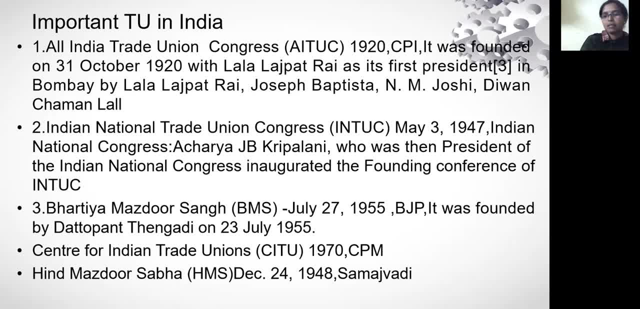 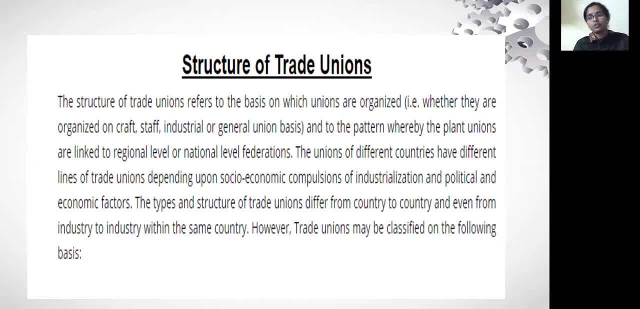 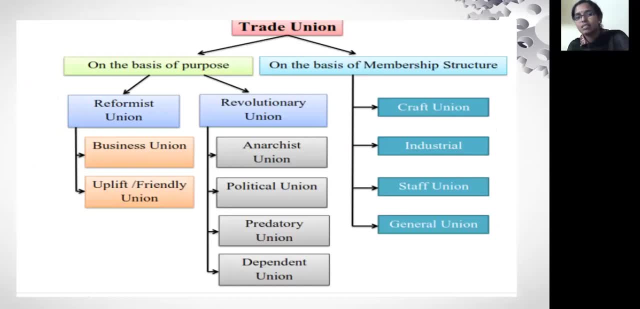 HMS Hind Masjid Sabha, formed in December 1950. And the political party- influence of the political party- is Samajwadi Party. So now we'll go through. structure of trade unions. a small glance of the structure of trade unions. So the structure of trade unions- see the trade unions- has been formed. 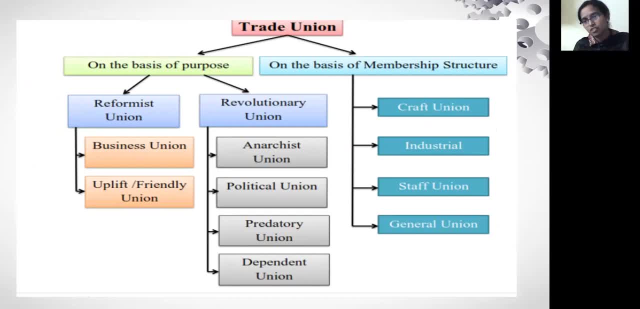 on the basis of purpose and on the basis of structure, membership structure. So again on the basis of structure, these trade unions has been again formed in into two types. One is reformist trade union, reformist unions and revolutionary unions. Let us see reformist unions and then we'll go through revolutionary unions. See the classification. 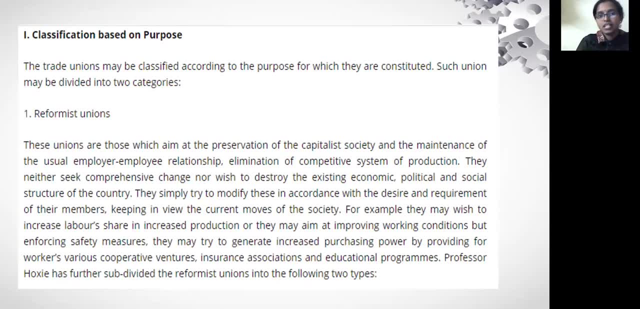 based on the purpose. The first one. the trade unions have been classified according to the purpose for which they are constituted. Such unions may be categorized into two unions. One is reformist unions and revolutionary unions- Reformist unions generally. these unions. 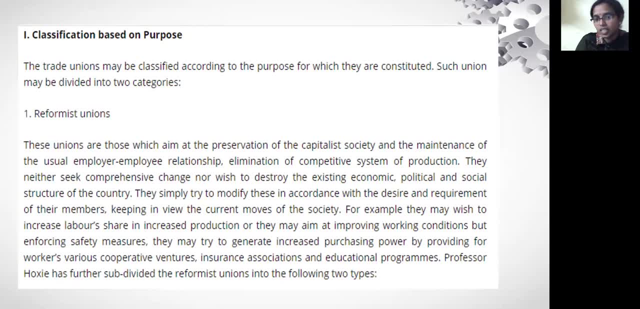 the aim of these unions is to preserve the capitalist society and to maintain the usual employer and employee relationship. They don't want to eliminate the competitive system of production. They don't want to disturb any competitive system of production. Neither they want to see comprehensive change, nor they. 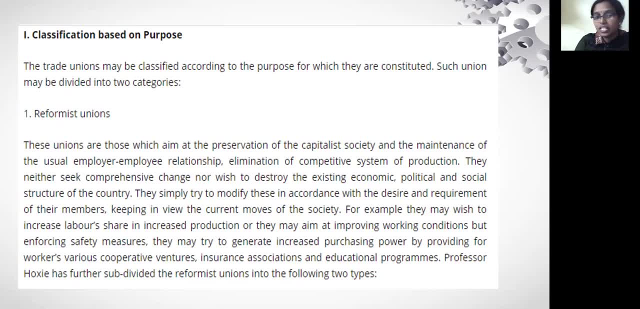 want to destroy the present economic, political and social structure of the country. they just want to have a, maintain a relationship. okay, they don't want to disturb and they want to. they simply modify in according to the desire and requirement of their members, keeping in you the current movements of the 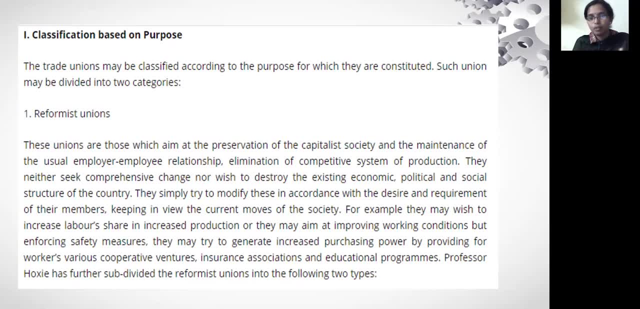 society in accordance with the society, economical, a political influences say this union will be moving, they never. the aim is to preserve a capitalist society and to maintain usual relations between the employer and the employer, employer and employee. so they don't want to disturb a capitalist society. this is. 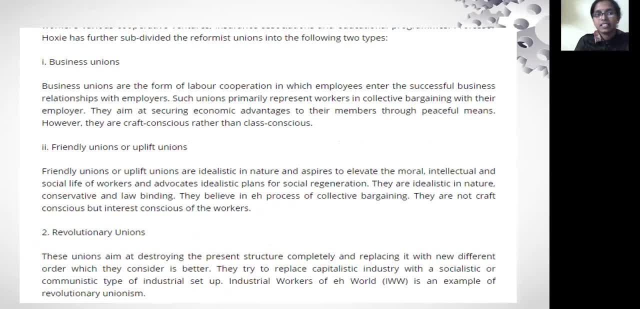 the reformist Union and- and next is Hoxsey- has subdivided it. this reformist union has been again subdivided into two different unions, that is, by Hoxsey and B Power union and friendly union, or this friendly union is also known as uplift union. friendly business unions are nothing, but they will be always thinking. 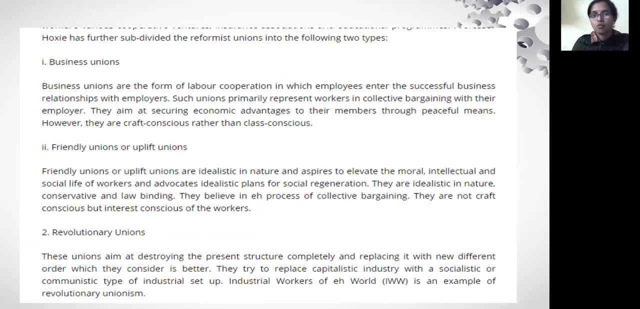 on an economic line. so they, always they aim. this union are formed is a form of lab of cooperation in which employees need the aid, enter into successful business relationship with the employers. they, their aim, is to enter into the business like only for the benefit of economic benefit, only for the economic 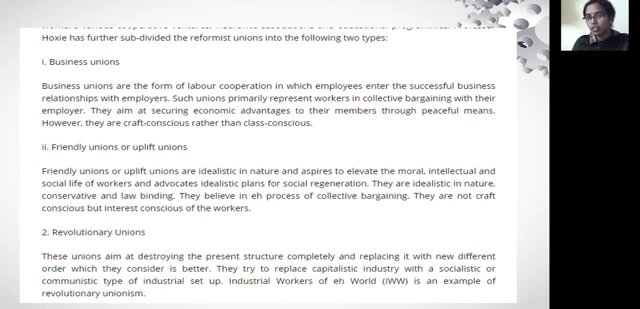 benefit such unions. they represent workers in collective bargaining with the employee. their aim is at securing economic advantage to their members through peaceful means. however, they craft consciousness, then class consciousness here. craft consciousness is nothing but crap. business conscience, economic conscious is more rather than class consciousness. business college. 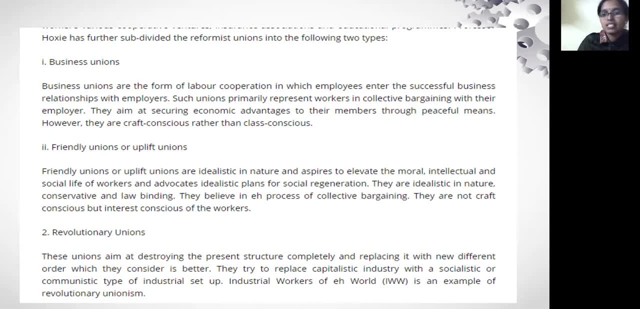 business business union and coming to the friendly union, this is quite opposite to the business union. these union will be having more class consciousness than that means they want to protect the interest of the workers rather than the economic benefit. rather than having an economic benefit, they want to concentrate on the benefit of the welfare of the workers. so that's why they are more class. 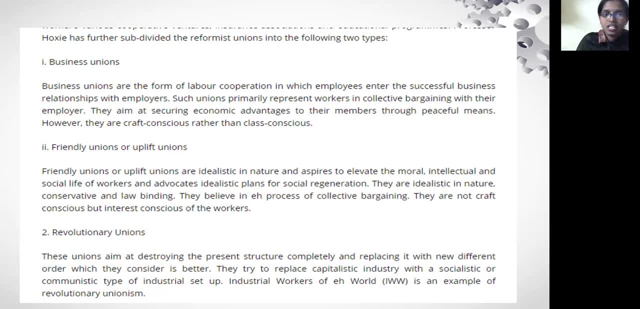 conscious than craft conscious. friendly unions are uplift unions are idealistic in nature. they are very noblistic in nature and aspires to elevate the moral, intellectual and social life of the workers and educate idealistic plans for social regeneration. this is one of the idle they'll be. 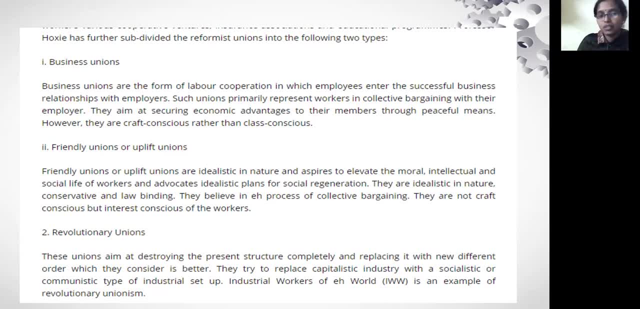 having. they'll be binding to this law, they'll be binding to the legal bonding. they'll be a social regeneration and they'll be believe in the process of collective bargaining and they are not craft consciousness but they are class consciousness. next is next type is revolutionary union. this is completely this type of union. is the these this type of union is they'll be having a 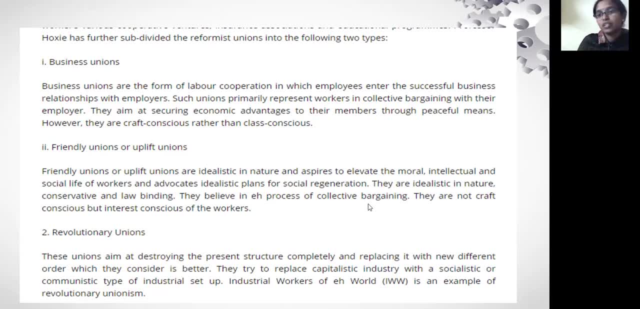 destroying. the aim of this type of union is destroying the present structure completely and replacing it with a different order which they consider it better. whichever is better they want to. they want to make a better structure by distracting or destroying the present existing structure. they try to replace the catholic society with a socialist or communist. 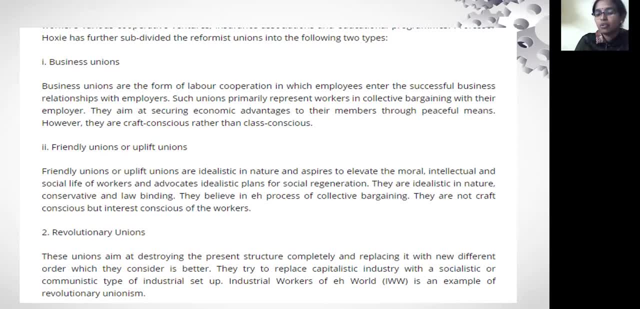 type of industrial setup. they wants to. they want to, they want to destroy the catholic type of society and want to replace this catalyst type of society with close to star communist type of industry setup. So, industrial workers, for example, this revolutionary unions has been formed during the 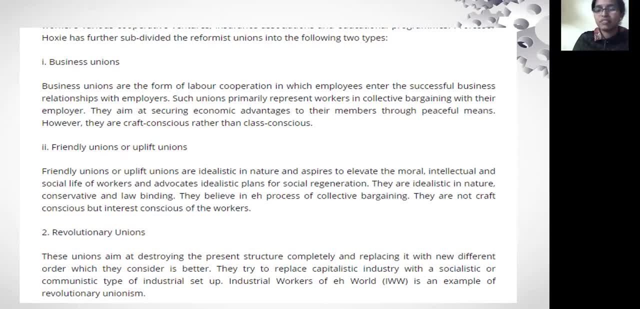 first world war one. So after the work of the world war one, with the deteriorating conditions, people were very much, very much inspired with inspired and they started revolting against the, against their exploitation of the workers, and they used to. they have started forming the revolutionary. 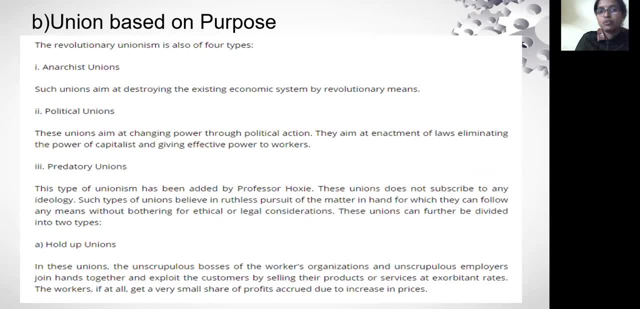 unions and their revolution unions, again divided into four types: anarchist, political unions, predatory unions and hold up unions. So the first one is anarchist unions. See, these anarchist unions are they'll having like. they want to completely destroy the existing system by revolutionary means. They want to destroy. the aim of this anarchist is. 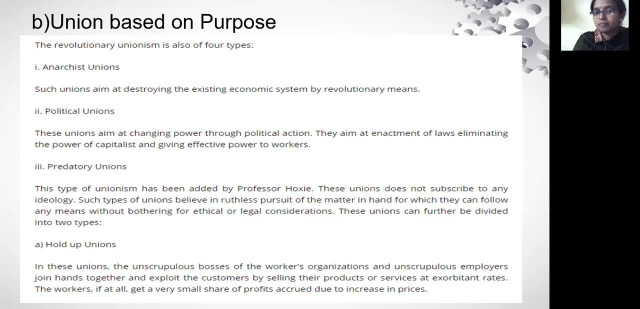 nothing but destroying the existing economic system and therefore by means of revolutionary means, and this political means. political unions are nothing but according to the convenience of the political party, power of capitalists and giving power to the workers. they here the political union. these union aim at changing the power through political action. 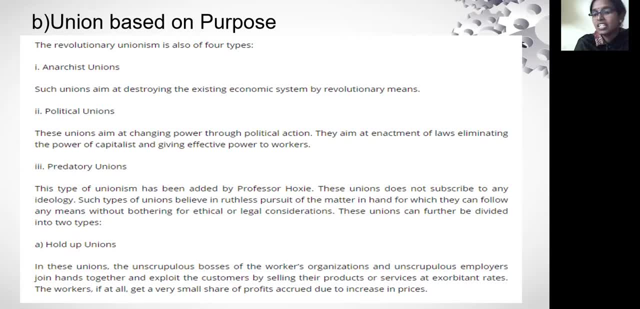 They. they want to change the power through the political action Here. the aim of this union is enactment of laws eliminating the power of capitalist and giving effective power to the workmen, and predatory unions. These type of unions have been added by Professor Hoxsey. These doesn't does not subscribe to any ideology. They don't. 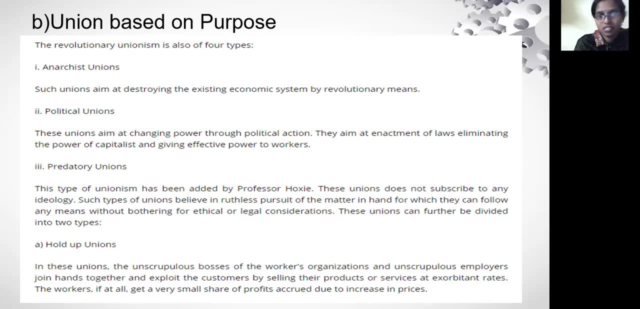 have any particular idea or they didn't have a prescribed or predetermined plan. They believe in ruthless pursuit of matter in hand, which they can follow by means of bothering ethical or without bothering about ethical or legal consideration. They'll just. they'll just like revolution, terrorism, terrorism, whichever they feel like. 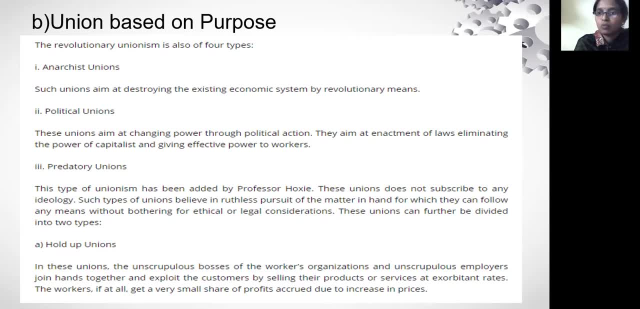 whether it is illegal or whatever the means, they'll follow the means to get what they want to get. So this type of union has been divided by Professor Hoxsey. These unions does not subscribe to any ideology. They don't have any particular idea to be followed. 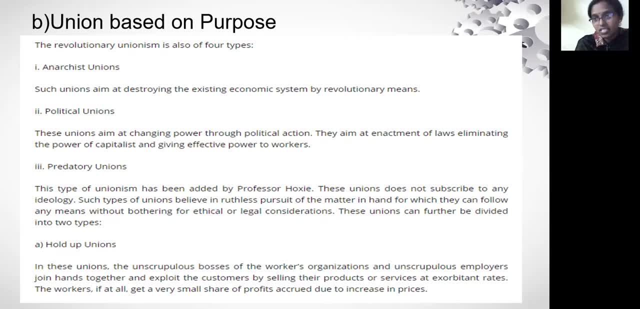 They'll be very rude and very revolutionary and hesitating minded. Whatever comes to your mind, what they want to achieve they'll achieve, and they don't know they don't follow a particular. they never bother about whether they are following your legal or method or ethical method or anything. 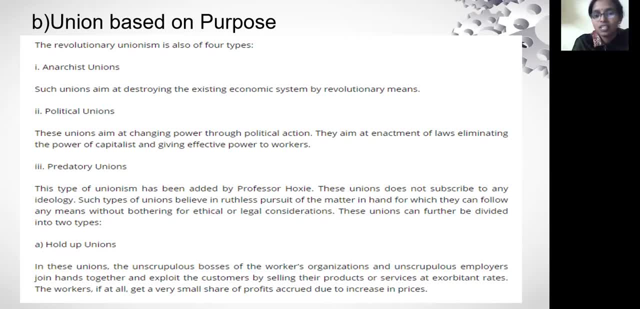 They never bother about that. They'll just be very ruthless, They'll be very rude and they'll follow illegal- consider illegal- lines to get what they want. So this has been again divided into hold up unions and gorilla unions. These hold up unions, these are like. 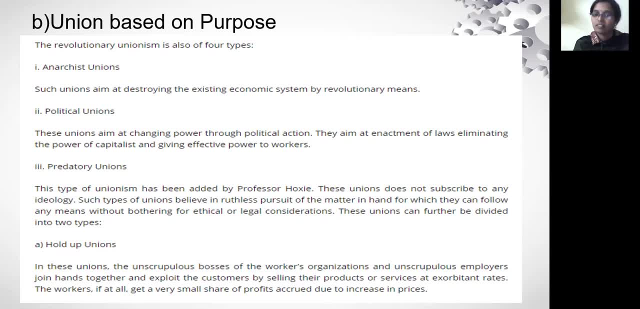 unethical, unfair bosses are of the organization. Unfair bosses are unfair employees, Unfair employers and unfair employees in the organization. they, they join hands together. They join hands together and they exploit the and exploit the customers by selling their products or the services at the exorbitant rates. 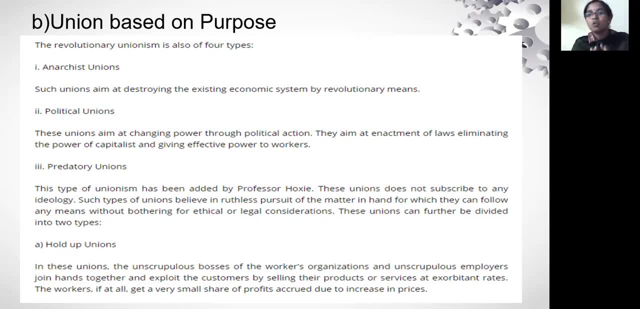 And they'll get the profits. So this is a hold up union, Hold up union, This union. what is that These people? they form into union? What? who are the representatives? The unsculptures means ruthless and unethical people, Unethical people. 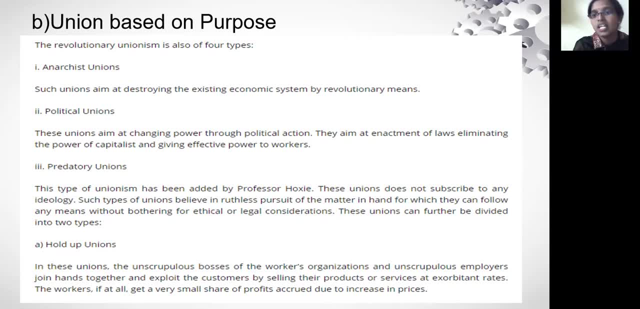 of the workers, among the workers and from the employers and employees they form into. they form into a group, and these they are unfair and rude. Okay, unfair and rude bosses of the workers organization and unfair and rude employers join together and they exploit the customers and they get the profits. 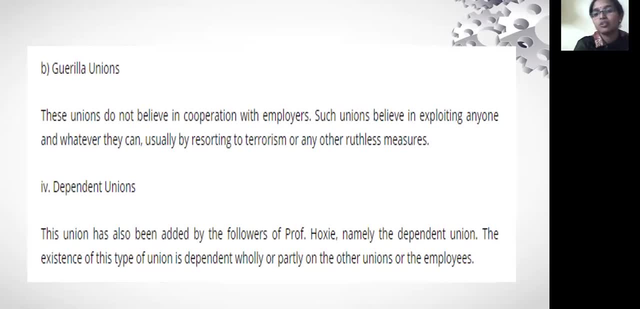 And the next is gorilla unions, which I said. they'll follow the ruthless measures to get whatever they want. So these unions do not believe in cooperation with the employers. They, they just operate opposite. They are, they are opposite with the hold up unions. In hold up unions they will be cooperating. They. 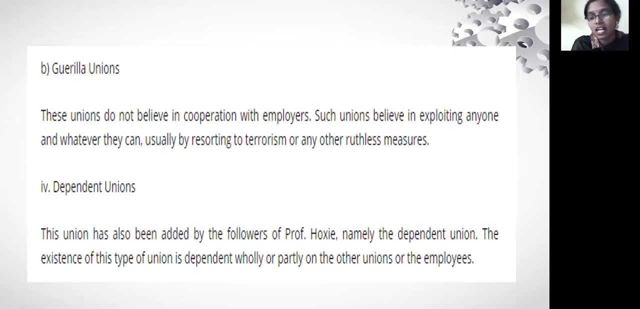 join hands with the employees. Employees and employers join hands together, Whereas here they won't believe in cooperation with employers. They believe in exploiting against anyone whatever they can do, like restoring to terrorism or any other ruthless measures, and they'll get whatever they want. 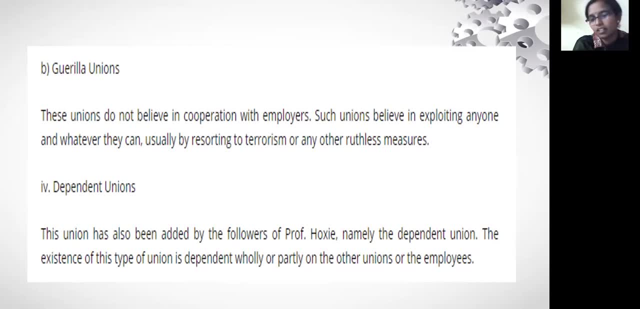 And dependent unions. these unions also been added by Professor Hoxsey and these existence of these unions is dependent wholly or partially on other you are unions or other employees. They'll be always depending upon the other unions or other employees Based on the membership, based on the 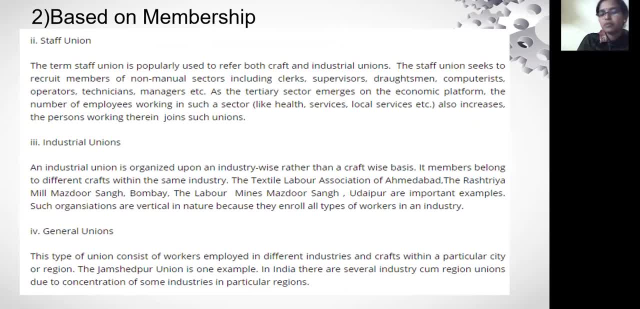 membership. it has been again divided into different types. One is craft union or staff union. The craft union- this is the one of the most popular union. The craft union- this is the one of the most popularly used report and this staff union and craft union seeks to 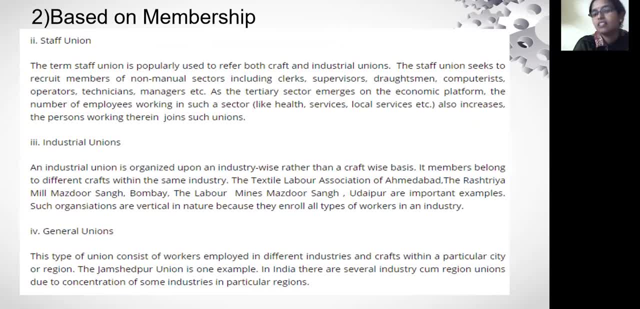 recruit members of non-mutual sectors like clerks, supervisors, draftsmen, computers operators, technicians, managers, etc. These territories manage to so like, for example, local services, health services. all these people form into a union. And then there's the skill union. 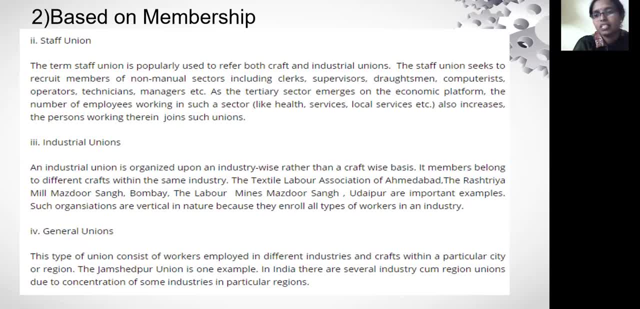 Skill union, technicians, operators- all these people form to a craft union And industrial unions. this is like industrial unions, like an industry union is organized upon industry-wise. Cotton industry, textile industry and the examples of the members belongs to different crafts. They belongs to like. 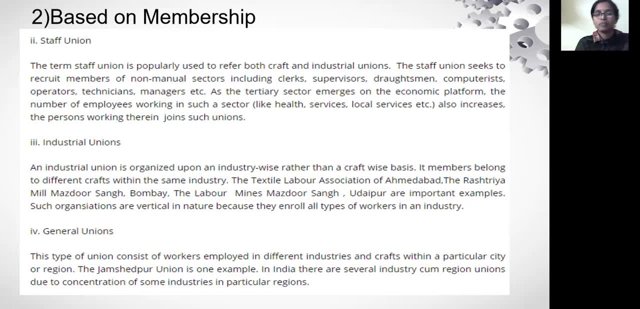 they'll form the industry-wide craft union. So they'll form the industry-wide craft union. So the industries from various textile industries, textile labo association of Amitabad, Rastriya mill, Mazur sangh, Bombay, and labo mines Mazur sangh, Udaipur, are the some of the important. 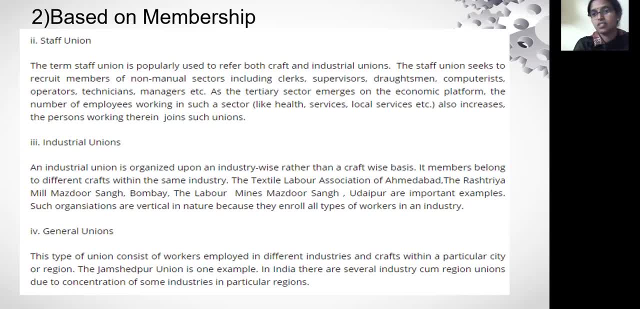 such organization, vertical in our nature, But they are all types of workers in the industries. So here what is happening? industry based upon the industry-wise. they will be forming into, Rather than craft, craftsmanship, the profession in this, in the first craft union or staff union they'll be forming, depending upon the 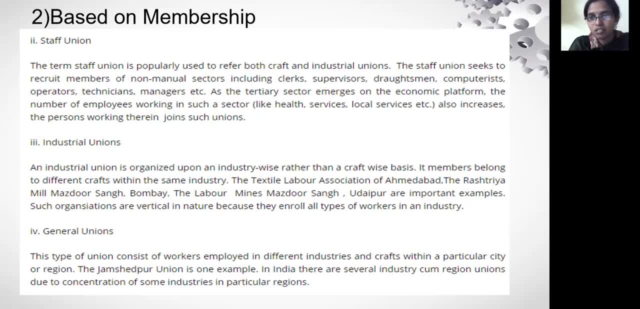 profession, like technicians, the computers, computer computers, clerks, into a separate union, whereas in the second industrial union they'll form into textile industry, software industry, or else oil industry, mines industry. they'll be forming into you, industry-wise they'll form into a separate union. coming to general union, these union consists, it doesn't have any particular 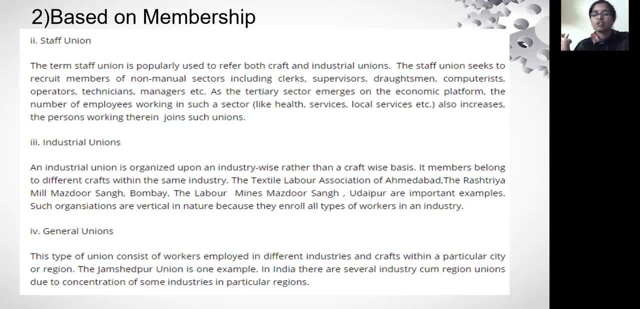 city or a region. the union consists of workers employed in different industries and different crafts. this is the combination of both the craft union and industrial union. in india there are several industry come region unions due to concentration of some industries in particular region and in india the trade unions will have been. 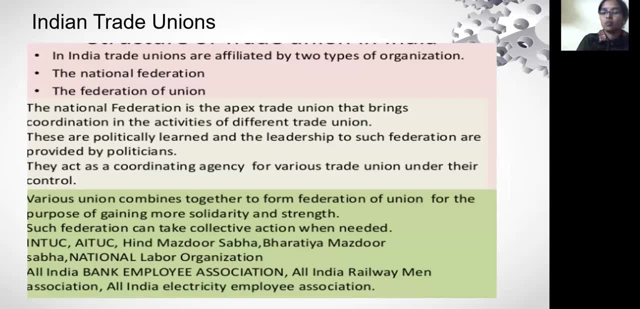 divided into two categories. one is they are affiliated to two different categories, that is, national federation and the federation of union. national federation is the epic body that belongs to cooperation in the activities of different trade unions. these are politically learned and the leadership to such federation are provided by politicians. totally it will. they will be controlled. 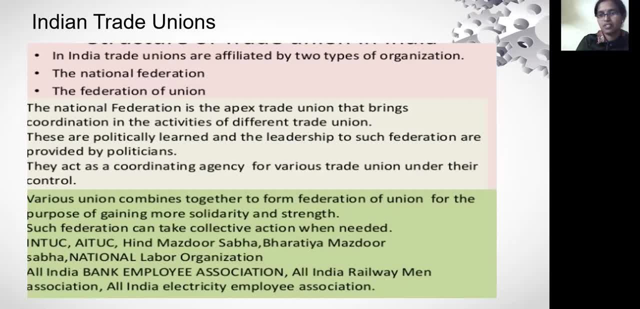 by the politicians. the first type sort of for national federation will be completely coordinated and controlled by the um national federal politicians, and the second one is the best example for of this is at the central level there will be um. various union combinations form into federation of unions for the purpose of gaining more solitary and strength at the 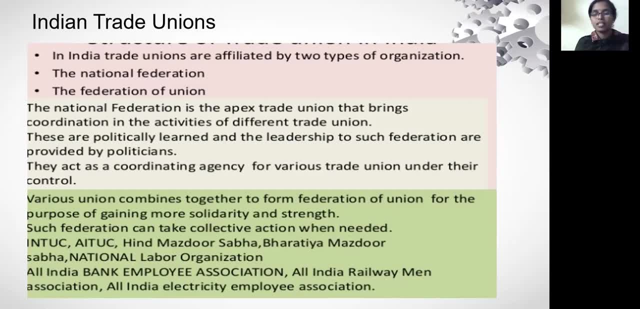 central level- uh, these are federal, federal unions will be taking place like aituc, intuc. all the central level unions come into. as an example of this: bank employee association, all the bank employees. all india railway men association, all railway workers in the country. all india electricity employee association. all india means all the worker electricity workers. 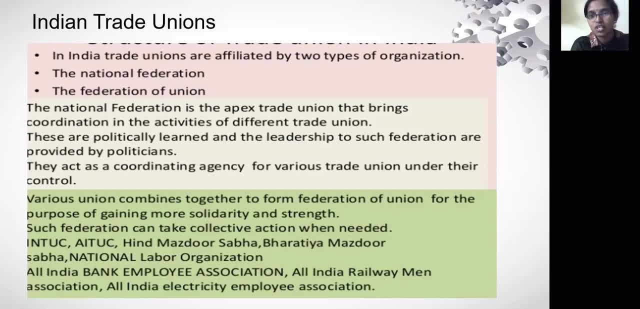 in in the country will be forming india association so as to have a solitary and rengiers association to to get the things, whatever they want to achieve, right. thank you very much for listening. in the next class we'll be looking into a more interesting topics like id act, industry dispute act and trade unions act, if 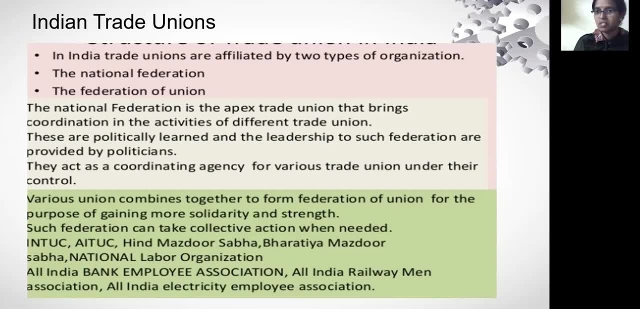 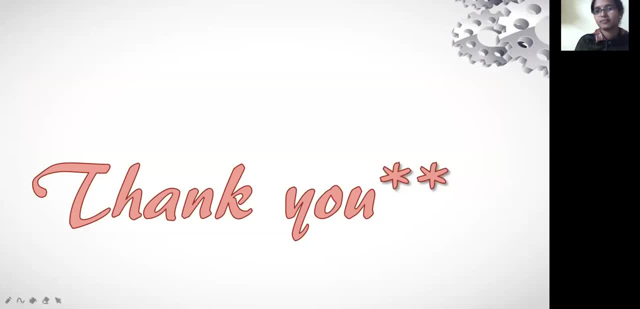 possible, we'll go through a collective bargaining, participatory management. thank you very much.